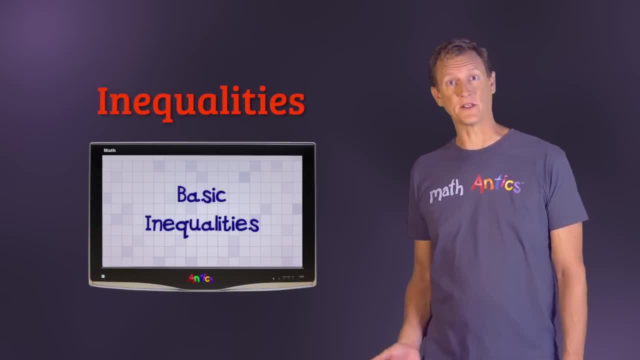 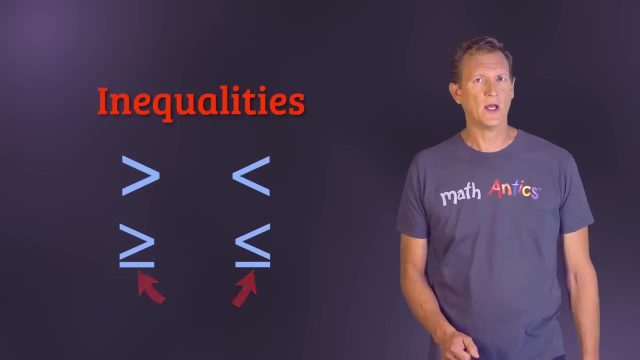 video- Basic Inequalities. Those sorts of comparisons use the greater than and less than signs, along with the versions of those that include the equal sign, And in this video I'm going to show you what happens when we use those signs. in algebraic equations Like the equation: 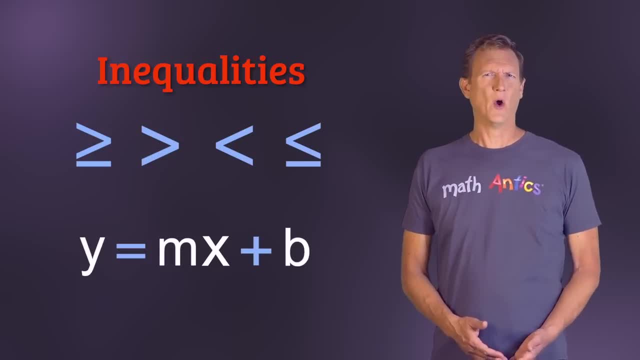 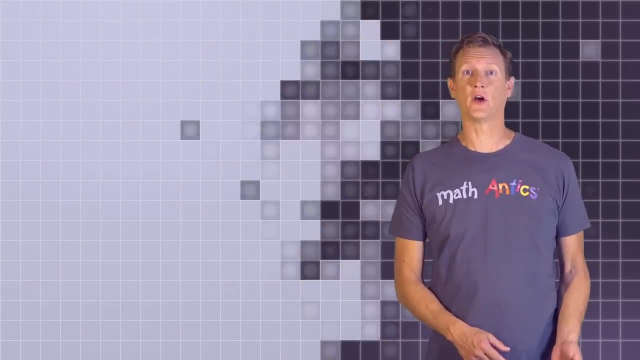 of a line: y equals mx plus b. What would it mean to have something like y is greater than mx plus b instead? To answer that question, let's first start with the very simple equation y equals x. If you watched our video called Basic Linear Functions- and I highly recommend- 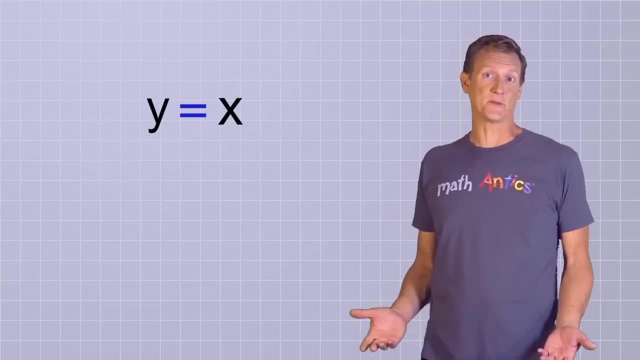 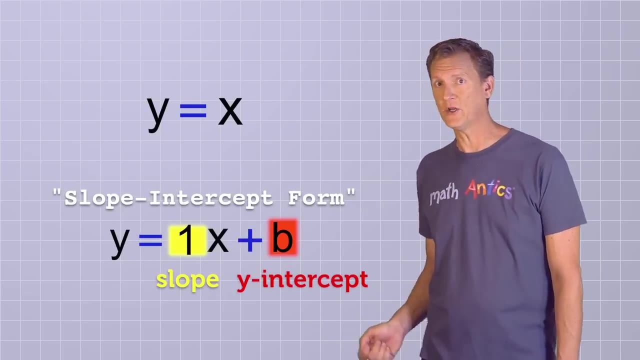 that you do, you'll remember that y equals x is just a special case of the slope-intercept form of a line where m the slope equals 1, and b the y-intercept equals 0. This equation tells us that whatever value x is, 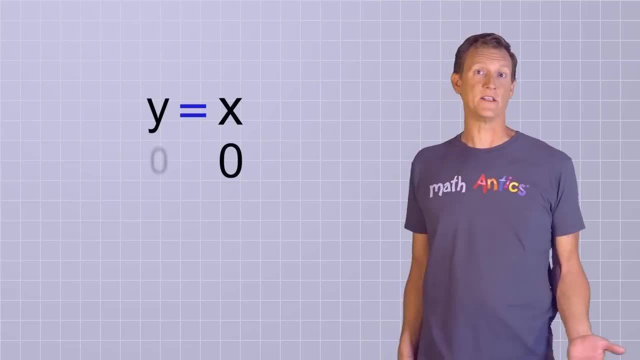 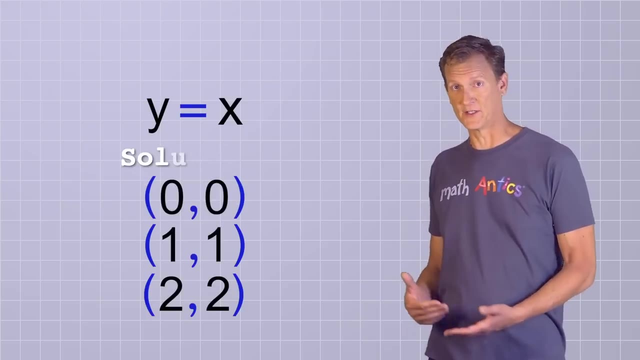 y must be the same. If x is 0, then y is 0.. If x is 1,, then y is 1.. If x is 2, then y is 2.. Every ordered pair- that's a solution for this equation- will have the same number. 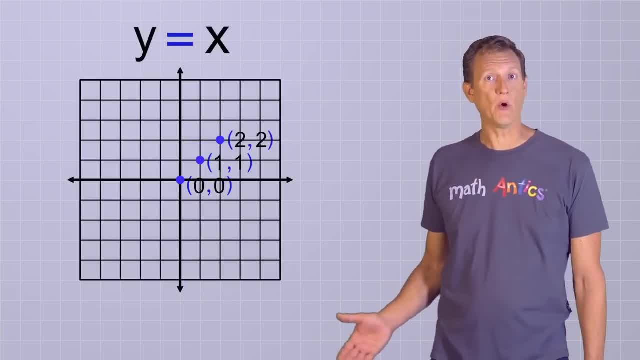 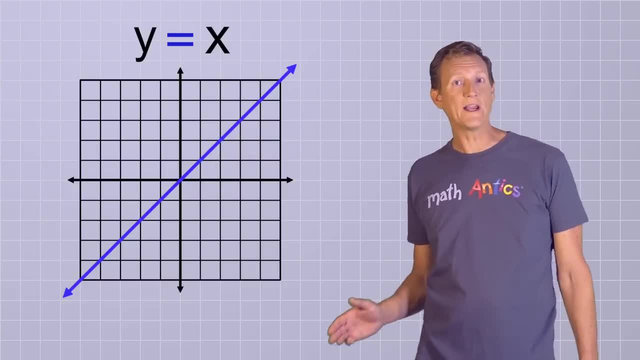 for y that it does for x. And if we graph some of those points on the coordinate plane, connecting the dots to show that there are infinite possibilities, we get a diagonal line that goes right through the middle of the quadrants 1 and 3.. 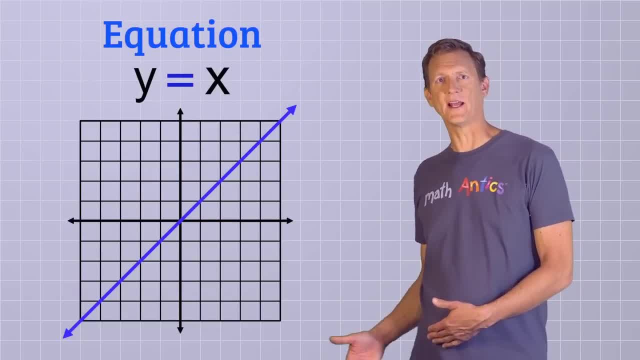 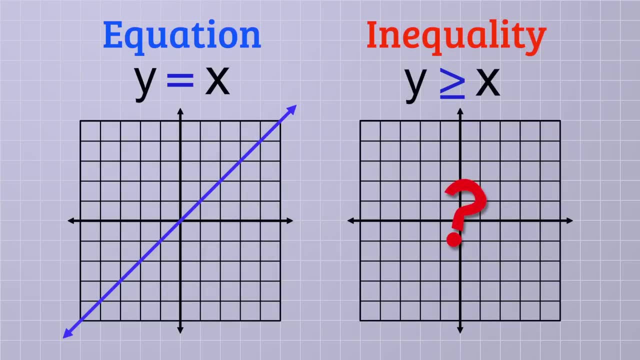 Now what if we change this from the equation y equals x to the inequality y is greater than or equal to x? How would that affect our graph? To figure that out, we need to determine all the combinations of x and y that would make this inequality true. 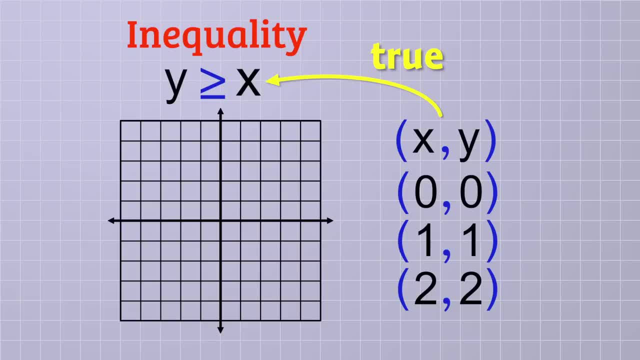 Well, fortunately, all of the solutions we found for y equals x will still work for this inequality, because it also contains the equal sign. That means that the diagonal line can stay in our graph, But the greater than sign opens up a lot of new possibilities. that would also make this. 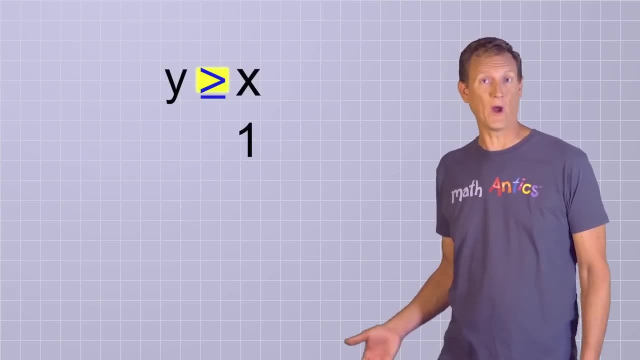 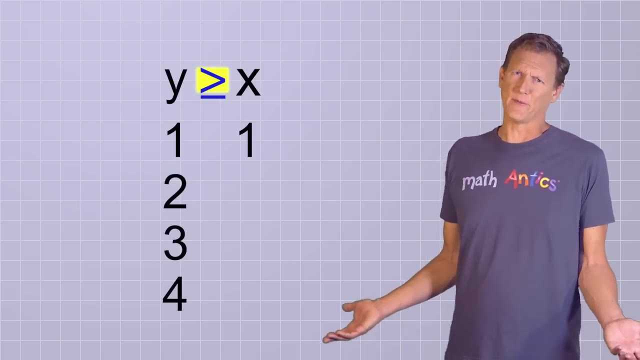 statement true. For example, if we let x be 1, y could still be 1,, but it could also be any number that's greater than 1, like y could be 2, or 3, or 4,, just to name a few. 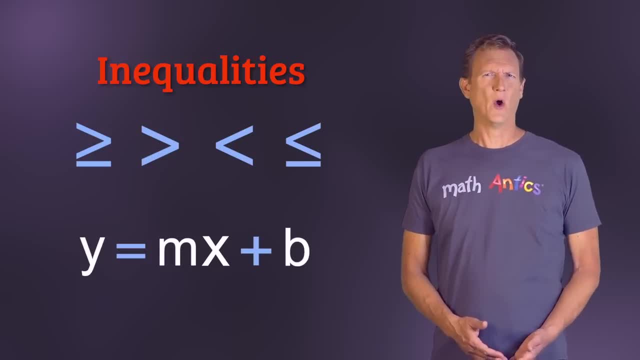 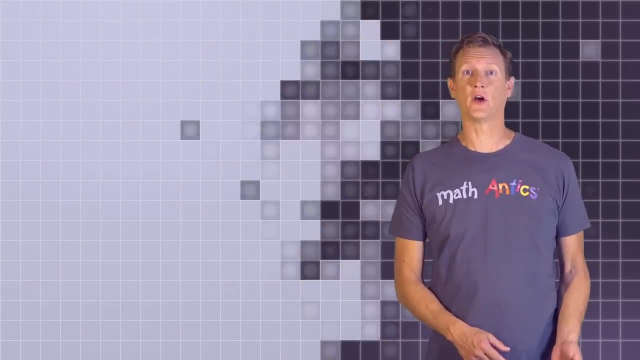 of a line: y equals mx plus b. What would it mean to have something like y is greater than mx plus b instead? To answer that question, let's first start with the very simple equation y equals x. If you watched our video called Basic Linear Functions- and I highly recommend- 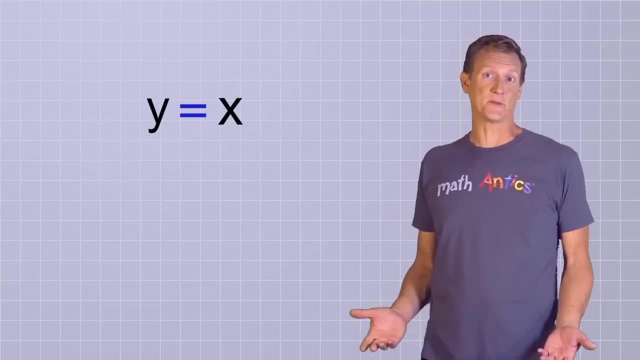 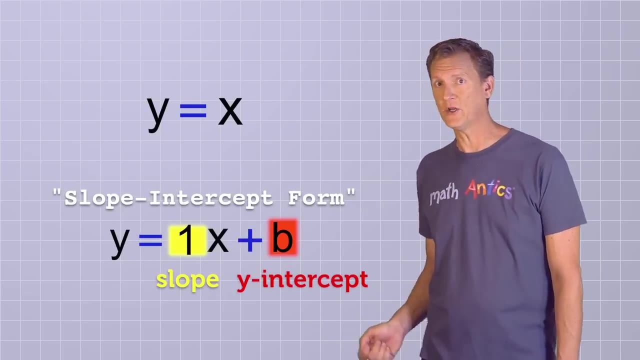 that you do, you'll remember that y equals x is just a special case of the slope-intercept form of a line where m the slope equals 1, and b the y-intercept equals 0. This equation tells us that whatever value x is, 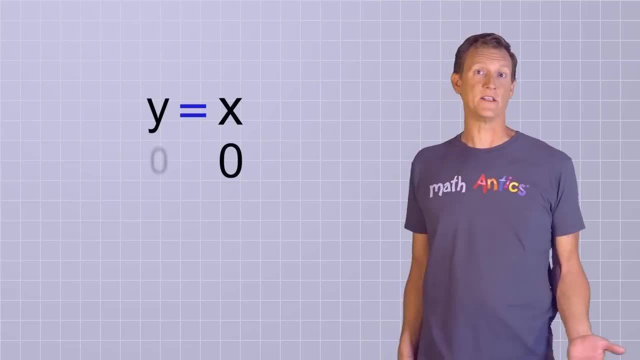 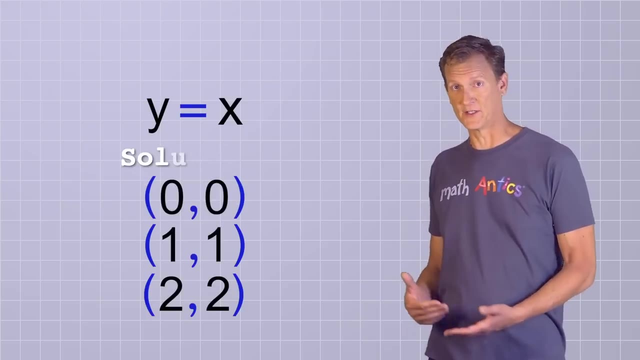 y must be the same. If x is 0, then y is 0.. If x is 1,, then y is 1.. If x is 2, then y is 2.. Every ordered pair- that's a solution for this equation- will have the same number. 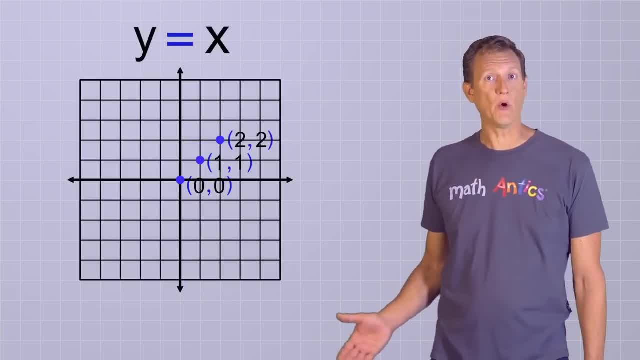 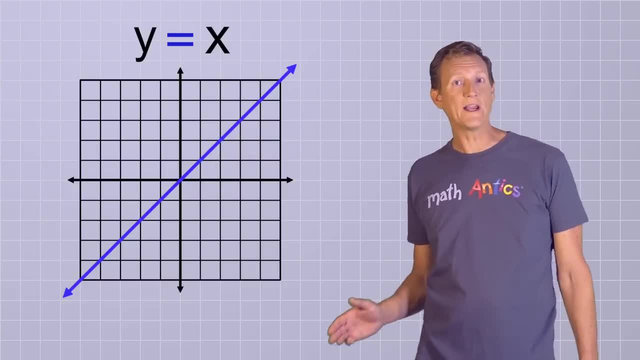 for y that it does for x. And if we graph some of those points on the coordinate plane, connecting the dots to show that there are infinite possibilities, we get a diagonal line that goes right through the middle of the quadrants 1 and 3.. 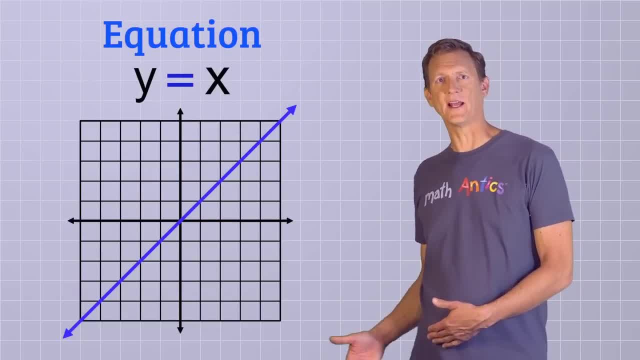 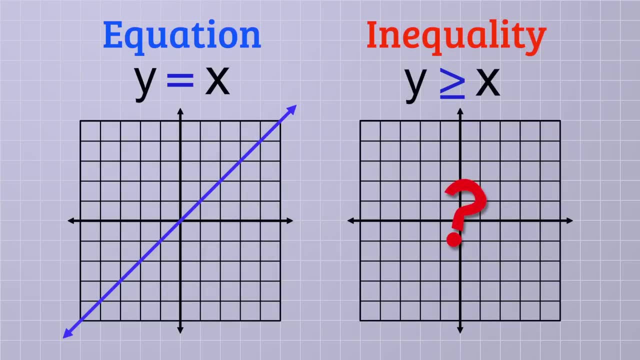 Now what if we change this from the equation y equals x to the inequality y is greater than or equal to x? How would that affect our graph? To figure that out, we need to determine all the combinations of x and y that would make this inequality true. 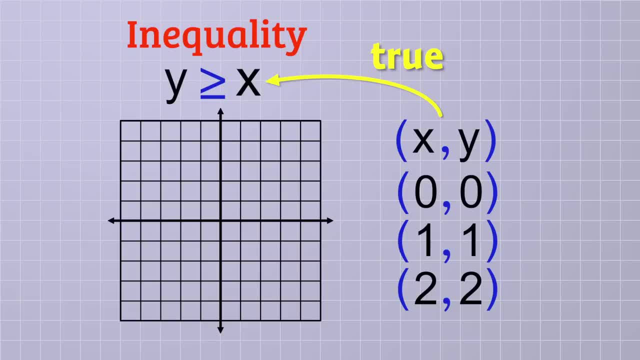 Well, fortunately, all of the solutions we found for y equals x will still work for this inequality, because it also contains the equal sign. That means that the diagonal line can stay in our graph, But the greater than sign opens up a lot of new possibilities. that would also make this. 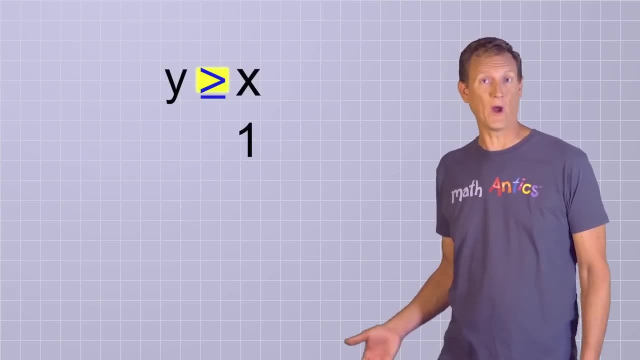 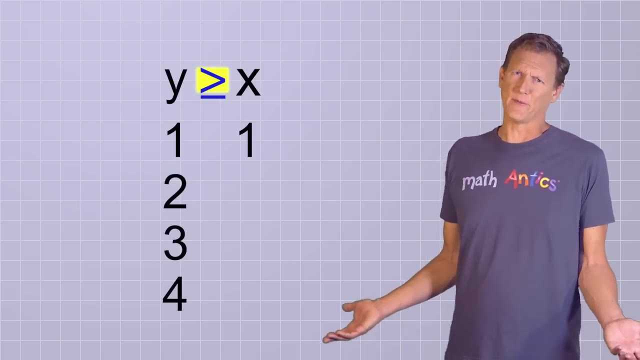 statement true. For example, if we let x be 1, y could still be 1,, but it could also be any number that's greater than 1, like y could be 2, or 3, or 4,, just to name a few. 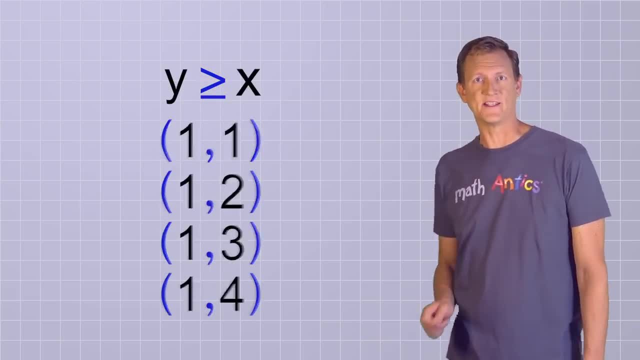 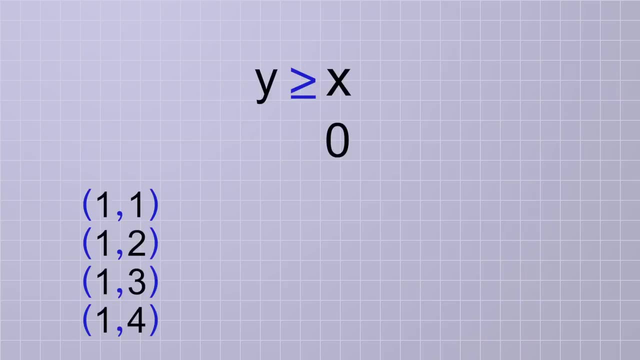 possibilities. Let's make ordered pairs out of those solutions and set them aside for a second. Then let's ask… Again, y could still be the same as x, 0, but it could also be any value greater than 0, y could be 1, or 2, or 3, and so on. Let's make ordered pairs from those also. 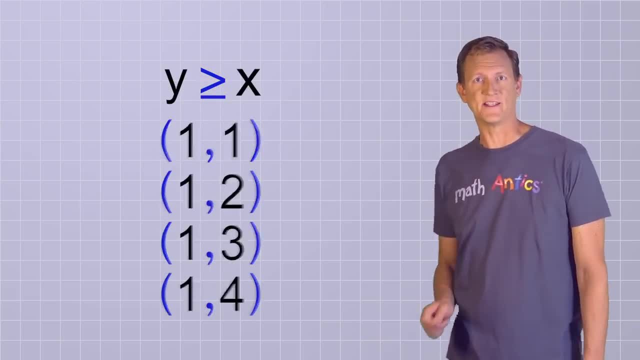 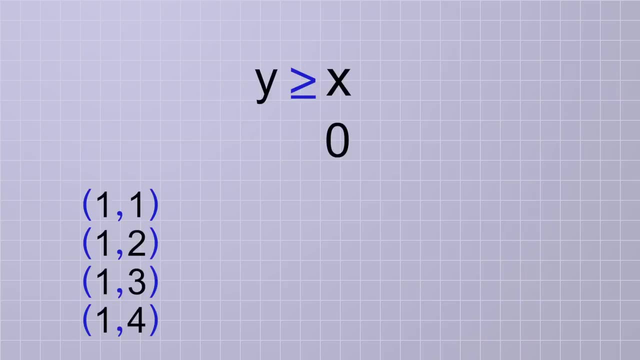 possibilities. Let's make ordered pairs out of those solutions and set them aside for a second. Then let's ask… Again, y could still be the same as x, 0, but it could also be any value greater than 0, y could be 1, or 2, or 3, and so on. Let's make ordered pairs from those also. 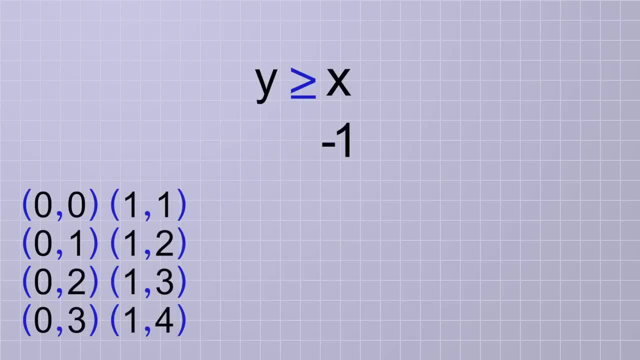 And then let's ask: what are some possibilities if we let x be negative 1?? In that case, y could be negative 1, or anything greater than negative 1,, like 0, or 1, or 2, and so on. 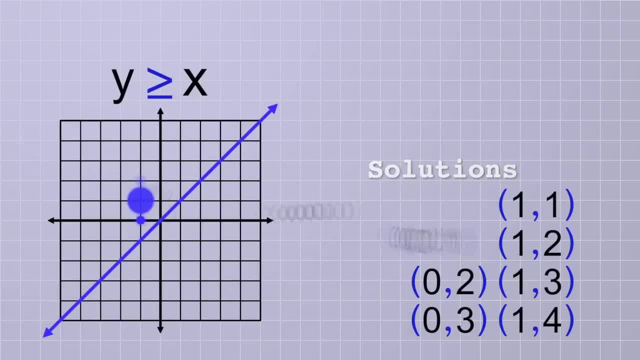 Now let's take these new solutions we've found and graph them on the coordinate plane. Do you notice that all of these new points are the same? All of these new points are above the diagonal line and none of them are below Any guess as to why. 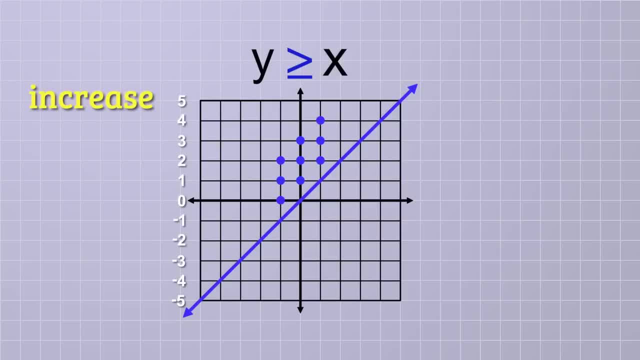 Yup, it's because on the coordinate plane y values increase as you go up and decrease as you go down. This diagonal is the y equals x line. right, Every point on the line has a y value that's exactly the same as its x value. That means that every point above 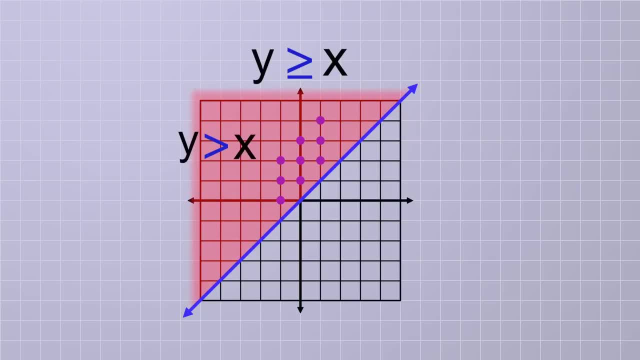 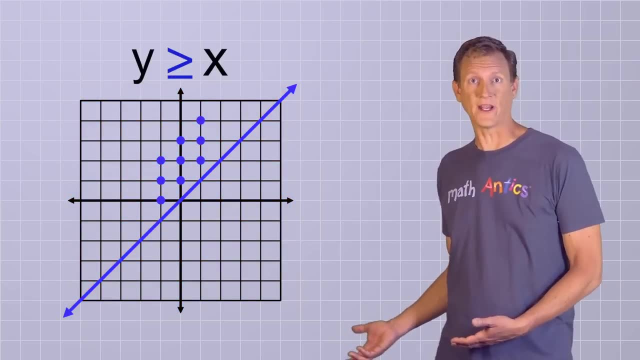 the line has a y value that's greater than its x value, while every point below the line has a y value that's less than its x value. In other words… In other words, the solutions to this inequality aren't limited to just the handful of ordered. 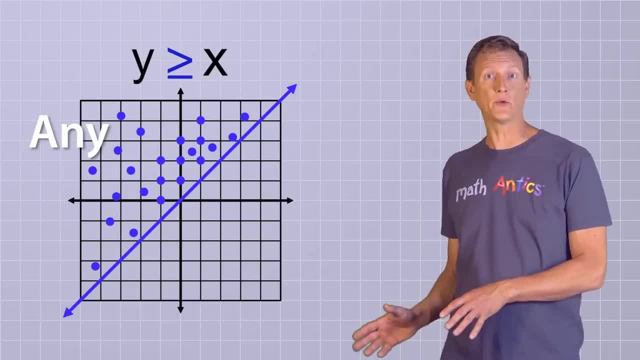 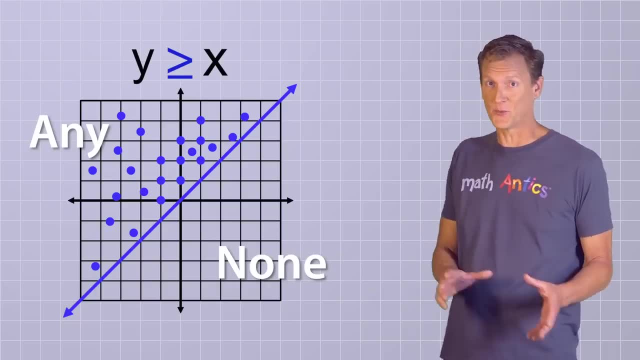 pairs we identified so far. Any point above the y equals x line would make the inequality true, but none of the points below it will To show that fact on our graph. since we can't draw an infinite number of points, the convention is to just shade in that area to cover all. 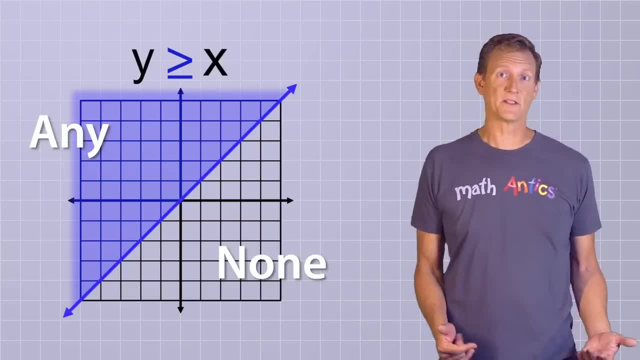 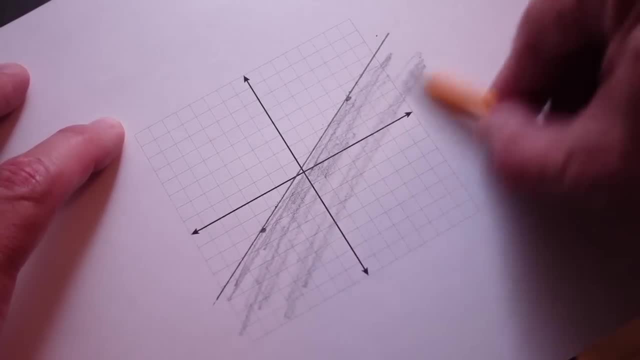 of them. Now, that's pretty easy to do with computer graphics, but there are also ways to do it on paper, with a pen or pencil. With a pencil, you can shade in large areas lightly by rubbing with the side of the pencil like this: With a pen, you can use a series. 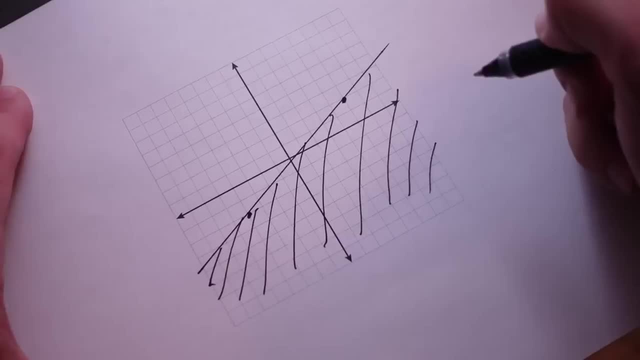 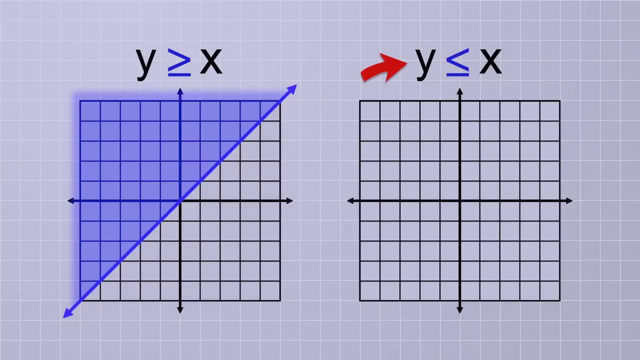 of lines or hatch marks to suggest that the whole area is included in the graph. Getting back to our digital graph, as you might expect, if our inequality had used the less than or equal to sign instead, then all of the solutions would be on or below the 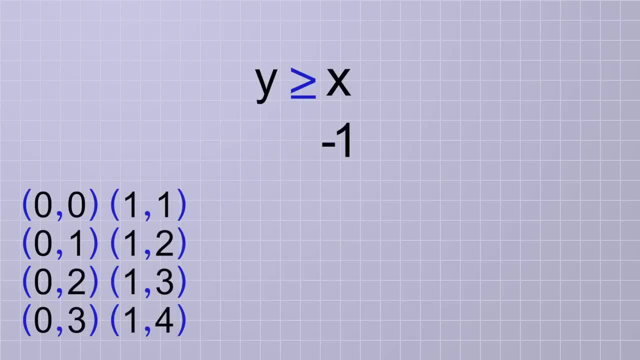 And then let's ask: what are some possibilities if we let x be negative 1?? In that case, y could be negative 1, or anything greater than negative 1,, like 0, or 1, or 2, and so on. 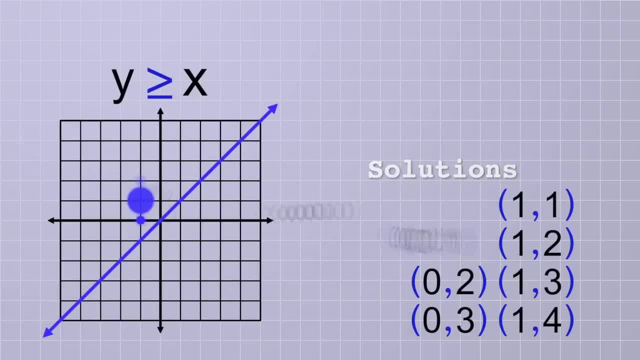 Now let's take these new solutions we've found and graph them on the coordinate plane. Do you notice that all of these new points are the same? All of these new points are above the diagonal line and none of them are below Any guess as to why. 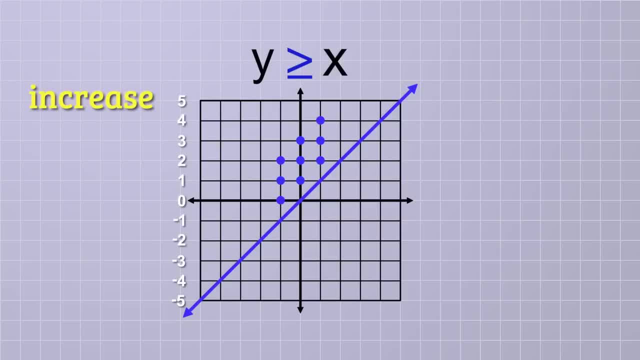 Yup, it's because on the coordinate plane y values increase as you go up and decrease as you go down. This diagonal is the y equals x line. right, Every point on the line has a y value that's exactly the same as its x value. That means that every point above 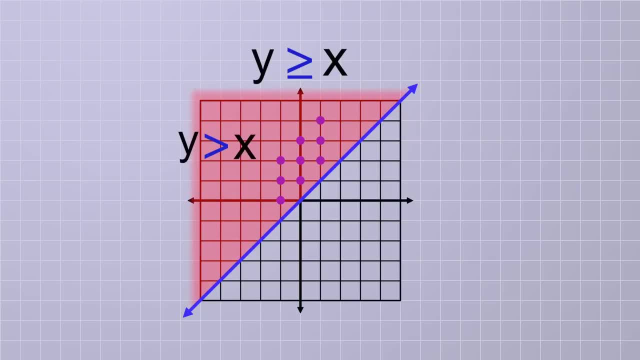 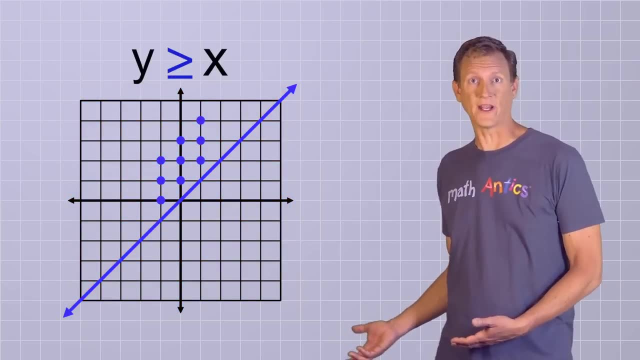 the line has a y value that's greater than its x value, while every point below the line has a y value that's less than its x value. In other words… In other words, the solutions to this inequality aren't limited to just the handful of ordered. 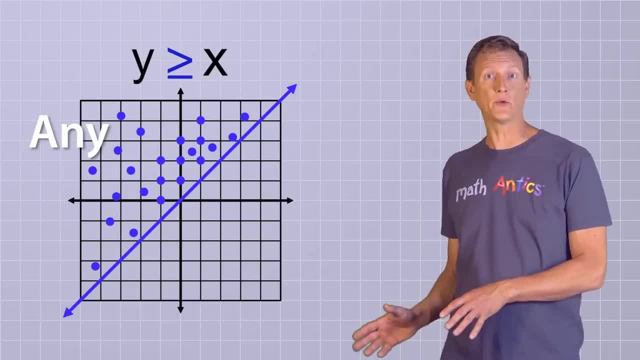 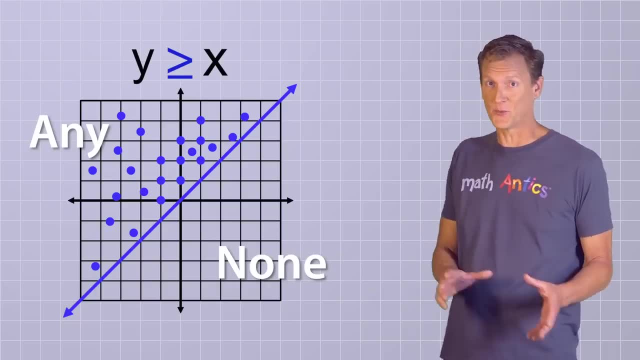 pairs we identified so far. Any point above the y equals x line would make the inequality true, but none of the points below it will To show that fact on our graph. since we can't draw an infinite number of points, the convention is to just shade in that area to cover all. 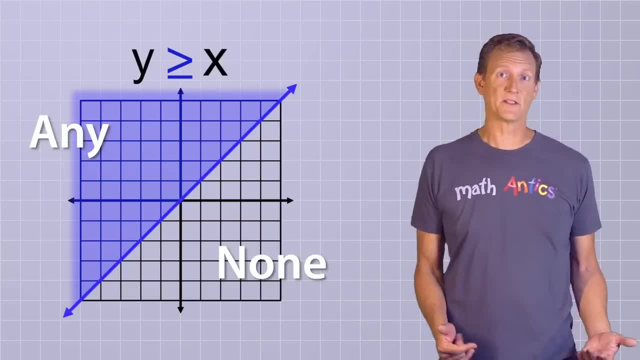 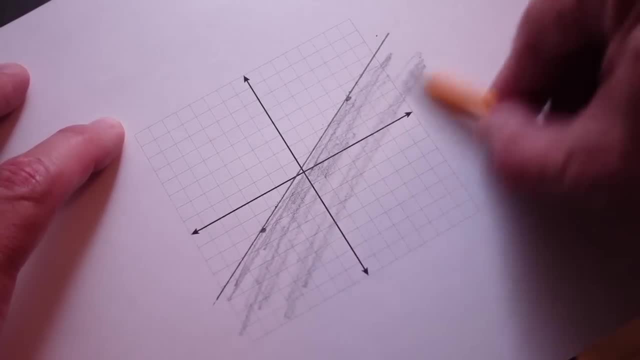 of them. Now, that's pretty easy to do with computer graphics, but there are also ways to do it on paper, with a pen or pencil. With a pencil, you can shade in large areas lightly by rubbing with the side of the pencil like this: With a pen, you can use a series. 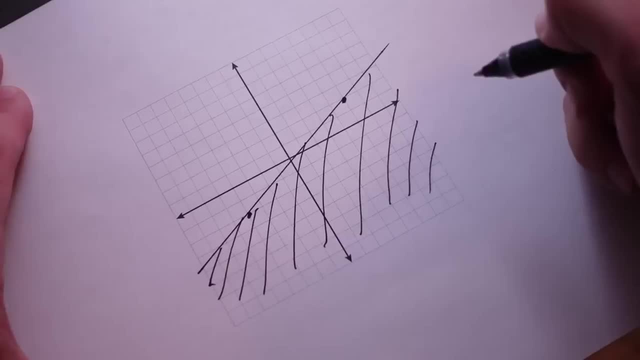 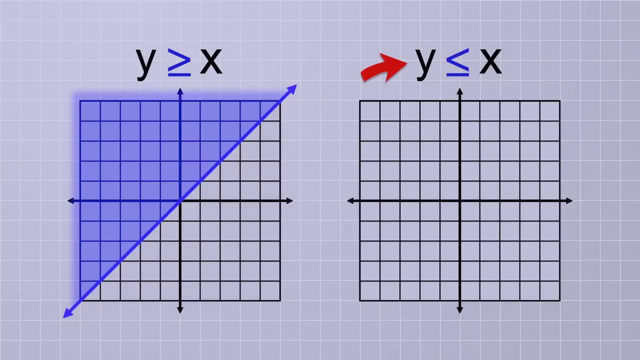 of lines or hatch marks to suggest that the whole area is included in the graph. Getting back to our digital graph, as you might expect, if our inequality had used the less than or equal to sign instead, then all of the solutions would be on or below the 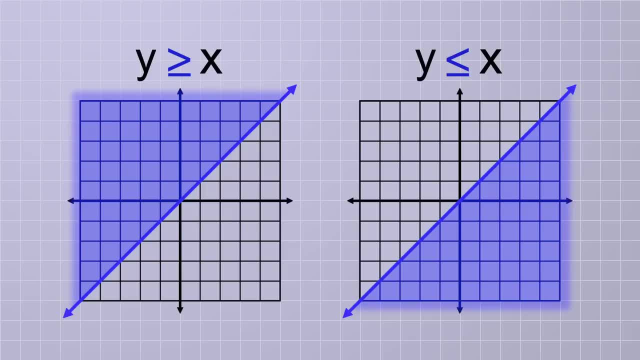 diagonal line like this: Because both of these inequalities include the equal sign, any point occurring directly on the y equals- x line is included in the set of valid answers. In fact, you can think of these inequalities like combinations of the equation y equals. 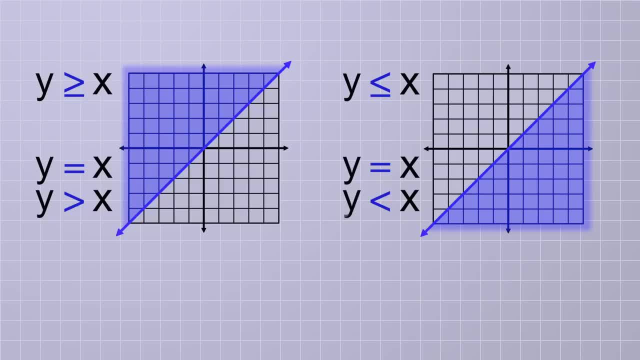 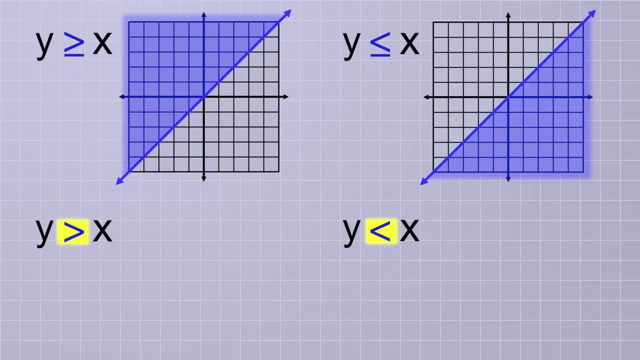 x and the inequalities y is greater than x and y is less than x. So what if we got rid of those equal signs and just used the pure greater than and less than signs instead? In those cases, none of the points exactly on the y equals- x line. 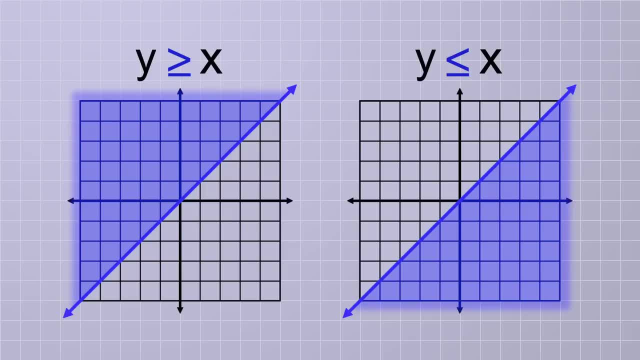 diagonal line like this: Because both of these inequalities include the equal sign, any point occurring directly on the y equals- x line is included in the set of valid answers. In fact, you can think of these inequalities like combinations of the equation y equals. 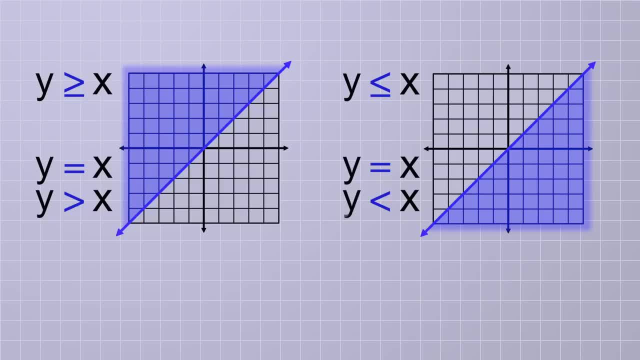 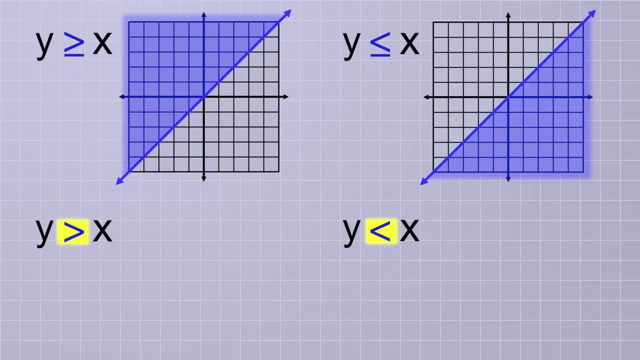 x and the inequalities y is greater than x and y is less than x. So what if we got rid of those equal signs and just used the pure greater than and less than signs instead? In those cases, none of the points exactly on the y equals- x line. 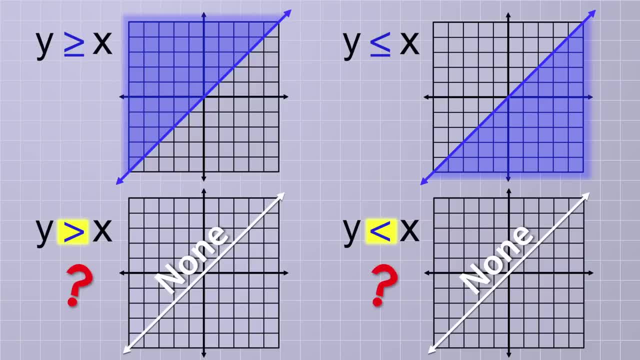 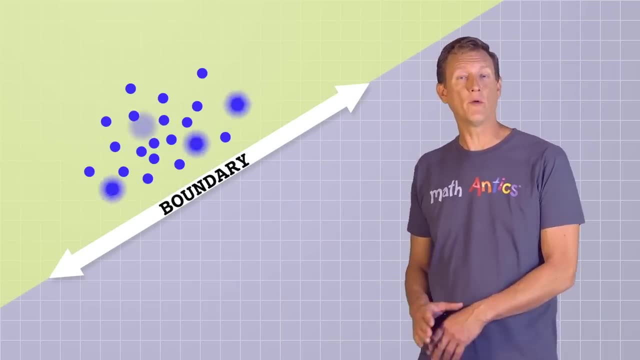 would be a solution to the inequality. But how can we show that on our graph? Well, the convention is to draw a solid line when the points exactly on the line are included, but draw a dashed line when they are not included. Basically, the line serves as a boundary On one side of it. all the points are definitely. 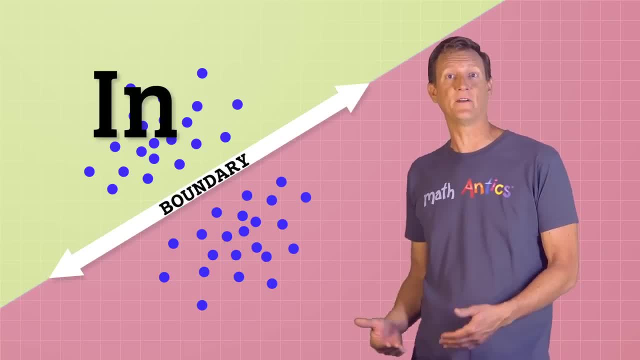 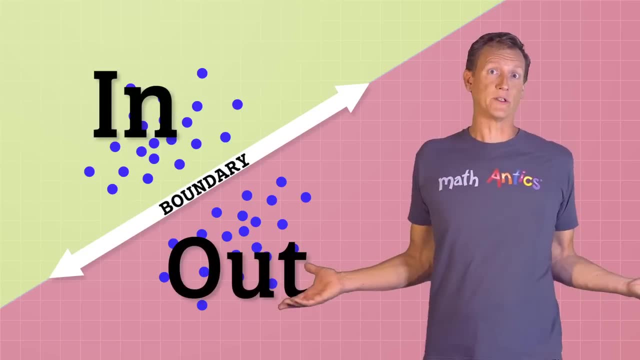 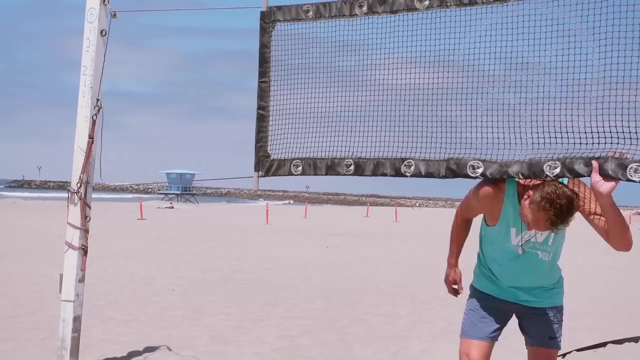 in the solution set and, on the other side, all of the points are definitely outside the solution set. As for the boundary itself, the question becomes: is the line in or out? Yes, Lines are out. My point: What are you talking about? Lines are out. 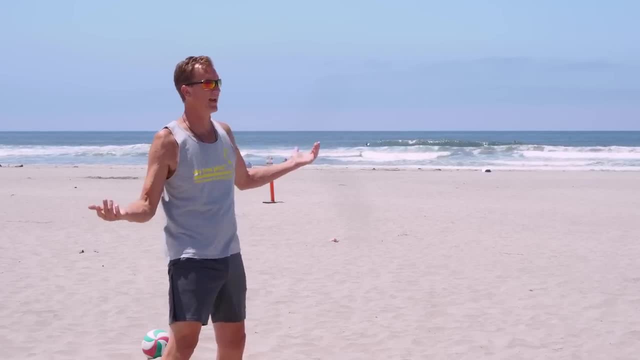 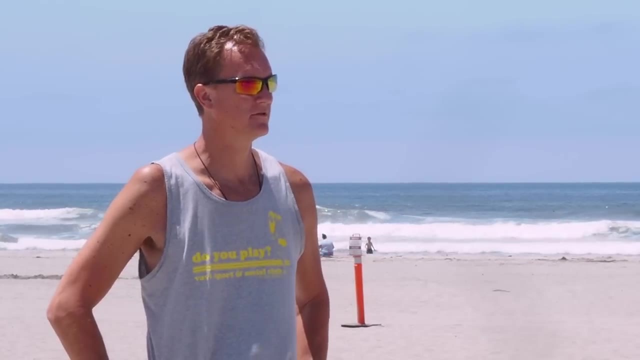 They're in. That's my point. Lines are out. Everyone knows that, Nuh-uh Well, if you're so sure, just look it up online. Alright, I will See. Lines are in. I suppose you believe everything on the internet. 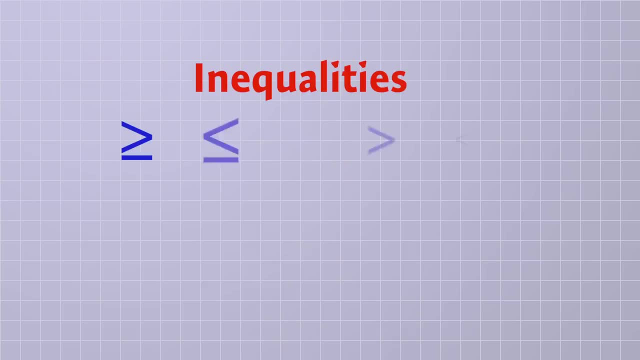 Fortunately, the rules for inequalities are easy to remember. If the inequality includes the equal sign, then the boundary line is in the solution set and you graph it with a solid line. But if it does not include the equal sign, then you draw a dashed line to show that the line is in the solution set. 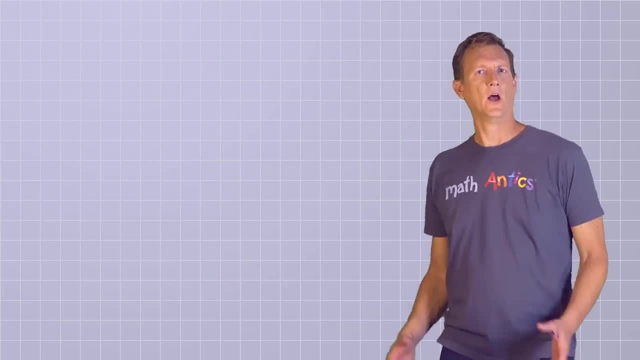 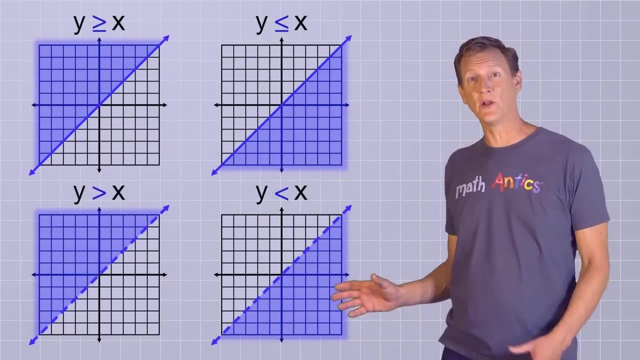 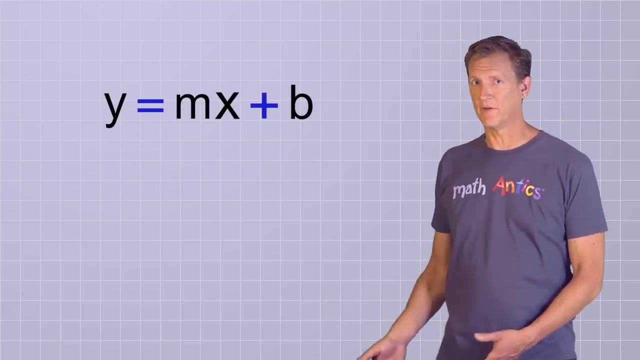 OK. so these four graphs should give you a pretty good idea how graphing inequalities works in general. But now we need to go beyond the simple y equals x equation to the general equation of a line. To do that, I'll walk you through the process of graphing the linear. 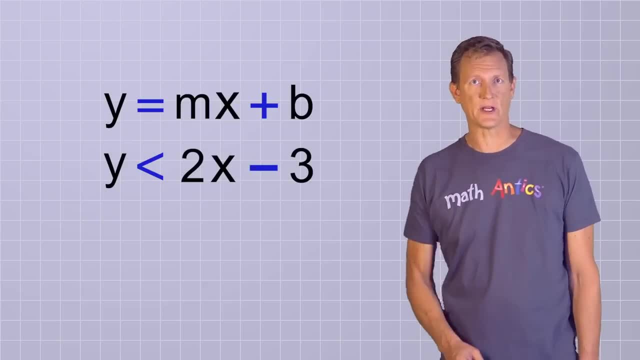 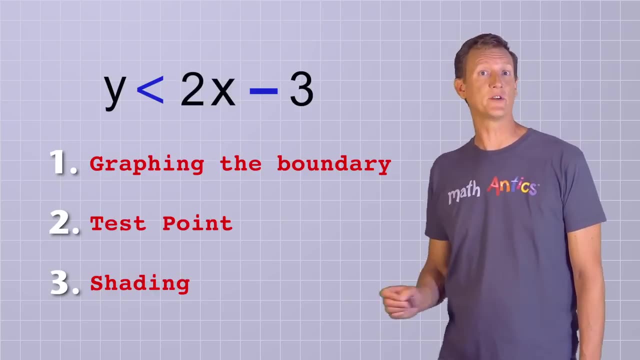 inequality y is less than 2x minus 3.. That will involve three main steps: Graphing the boundary line, picking a test point and shading the proper side of the line. Let's start with graphing the boundary line. To do that, first, pretend that the inequality 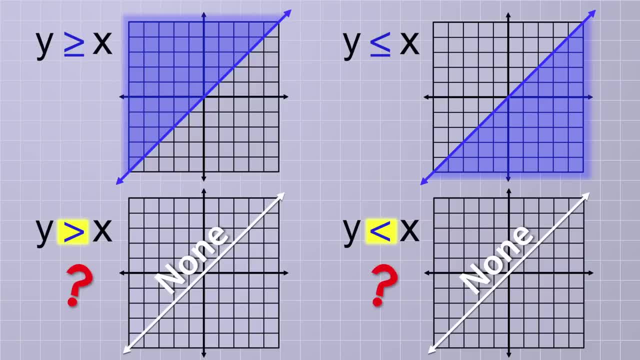 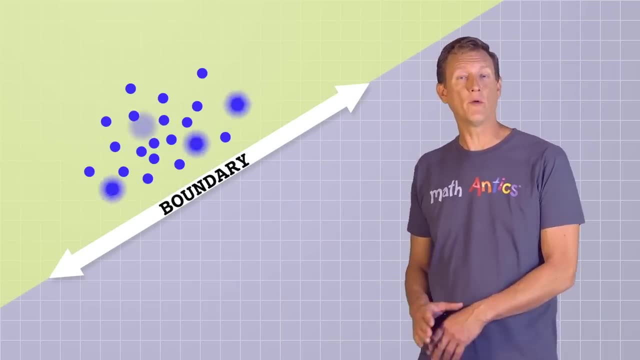 would be a solution to the inequality. But how can we show that on our graph? Well, the convention is to draw a solid line when the points exactly on the line are included, but draw a dashed line when they are not included. Basically, the line serves as a boundary On one side of it. all the points are definitely. 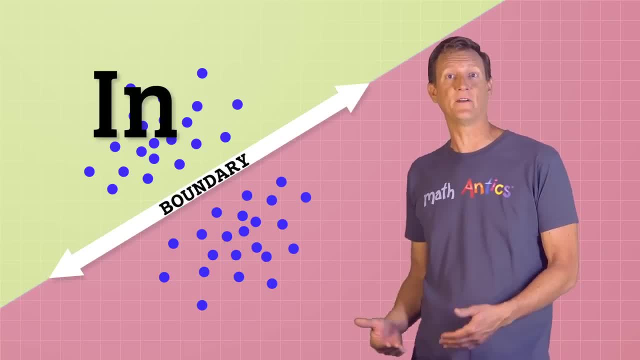 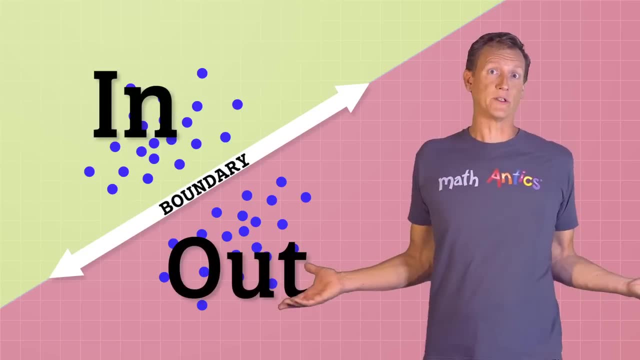 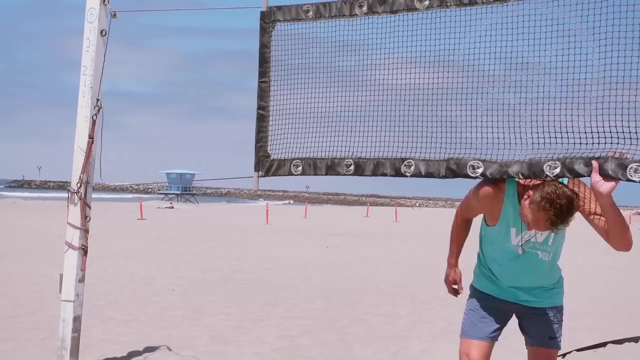 in the solution set and, on the other side, all of the points are definitely outside the solution set. As for the boundary itself, the question becomes: is the line in or out? Yes, Lines are out. My point: What are you talking about? Lines are out. 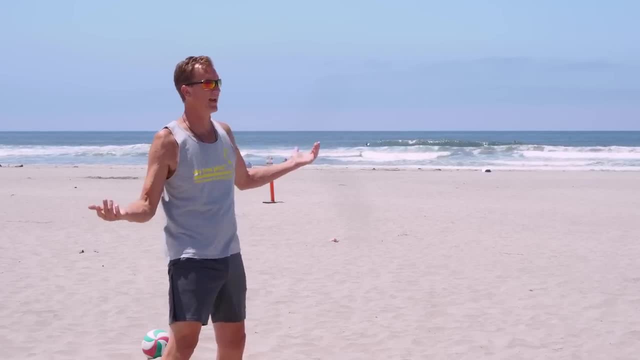 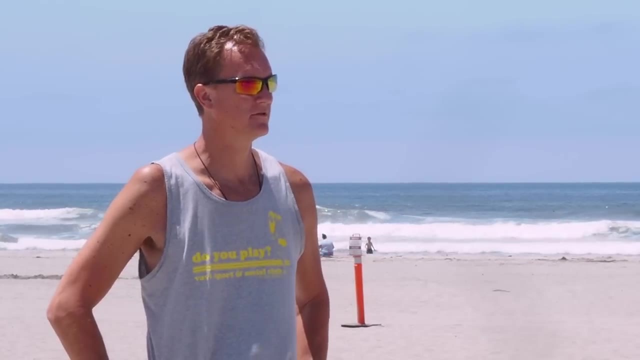 They're in. That's my point. Lines are out. Everyone knows that, Nuh-uh Well, if you're so sure, just look it up online. Alright, I will See. Lines are in. I suppose you believe everything on the internet. 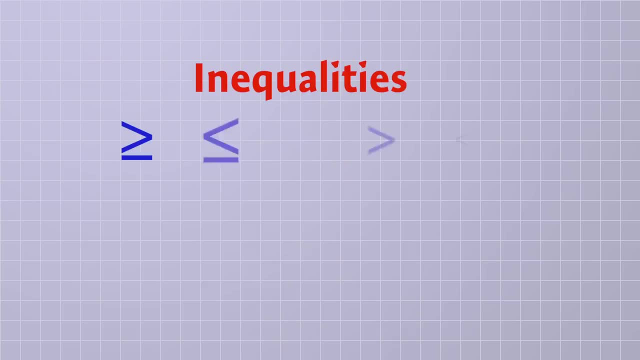 Fortunately, the rules for inequalities are easy to remember. If the inequality includes the equal sign, then the boundary line is in the solution set and you graph it with a solid line. But if it does not include the equal sign, then you draw a dashed line to show that the line is in the solution set and you graph it with a solid line. But if it does not include the equal sign, then you draw a dashed line to show. 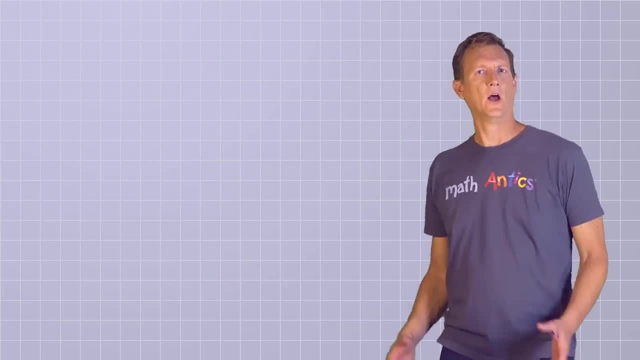 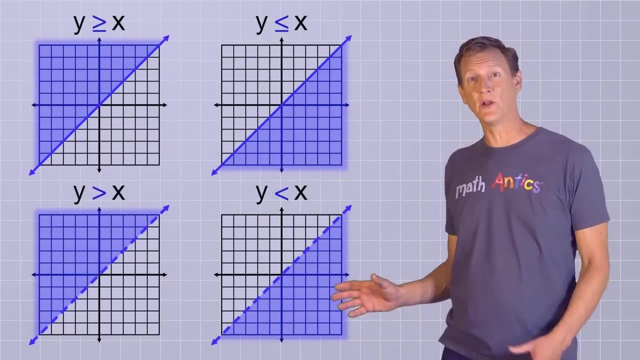 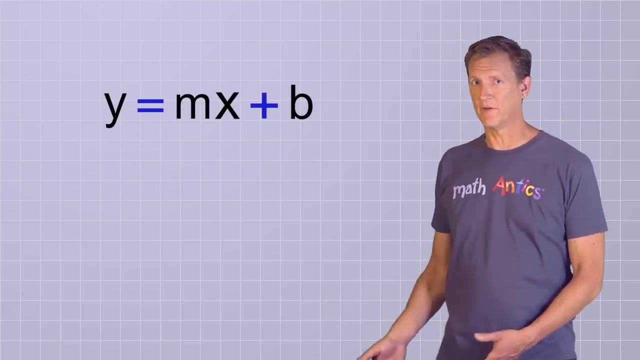 that the boundary line is NOT in the solution set. OK, so these four graphs should give you a pretty good idea how graphing inequalities works in general. But now we need to go beyond the simple y equals x equation to the general equation of a line. To do that, I'll walk you through the process of graphing the linear. 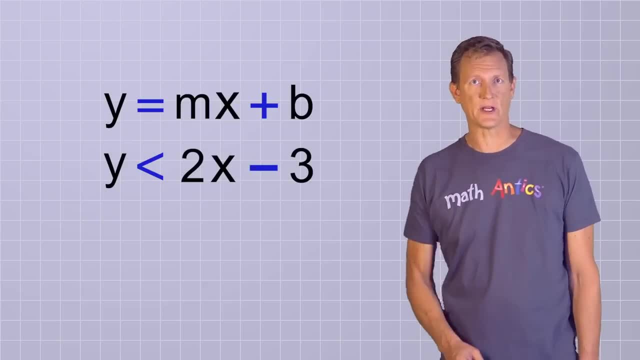 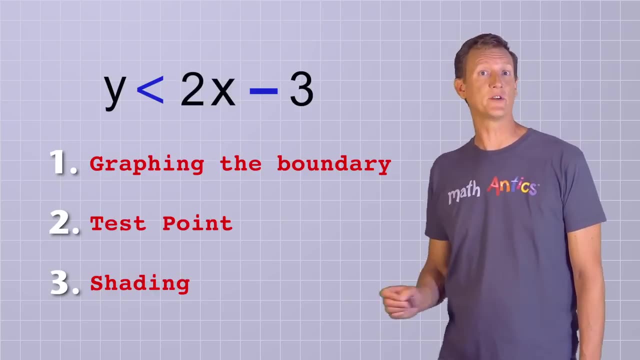 inequality y is less than 2x minus 3.. That will involve three main steps: Graphing the boundary line, picking a test point and shading the proper side of the line. Let's start with graphing the boundary line. To do that, first, pretend that the inequality 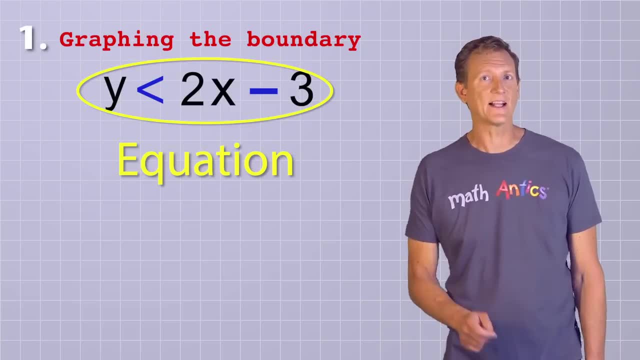 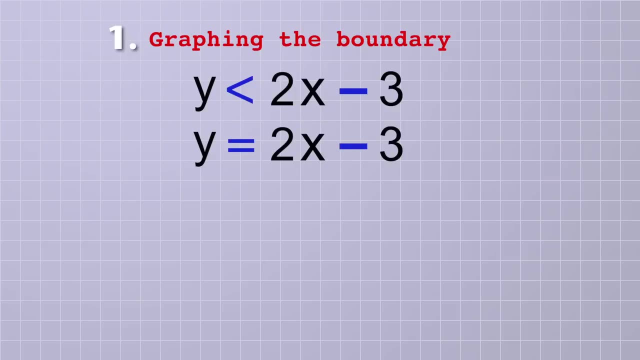 you have is actually an equation, so that you can graph it exactly the same way. you'd graph a line. That means rewriting it as y equals 2x minus 3.. To graph that line, we just need to plot any two points along it and connect the dots. 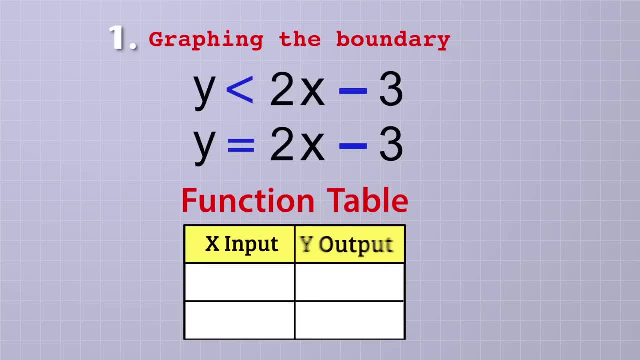 It's kind of like making a function table, but we only need to find the y output values for two different x input values. Any two points will do, so I'm going to pick x-input: x equals 2 and x equals negative 2, to keep things simple. 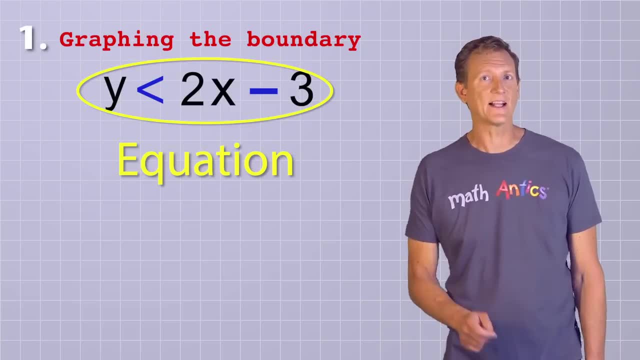 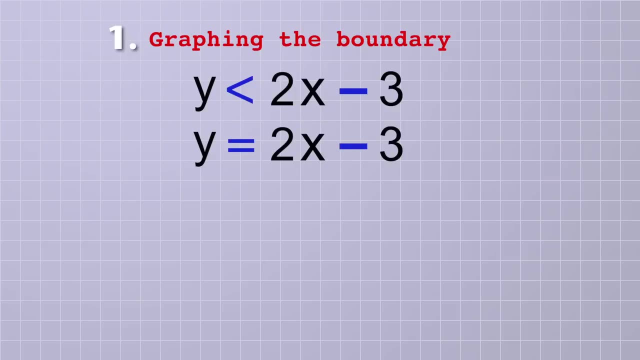 you have is actually an equation, so that you can graph it exactly the same way. you'd graph a line. That means rewriting it as y equals 2x minus 3.. To graph that line, we just need to plot any two points along it and connect the dots. 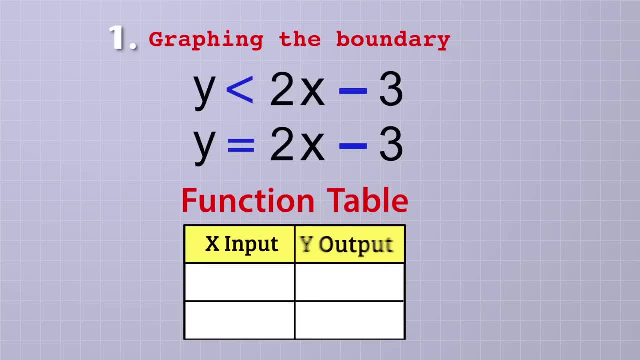 It's kind of like making a function table, but we only need to find the y output values for two different x input values. Any two points will do, so I'm going to pick x-input: x equals 2 and x equals negative 2, to keep things simple. 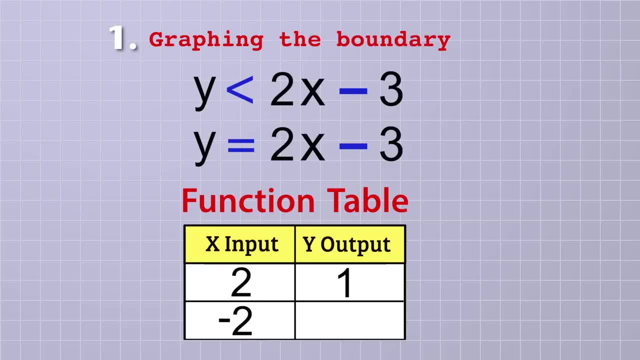 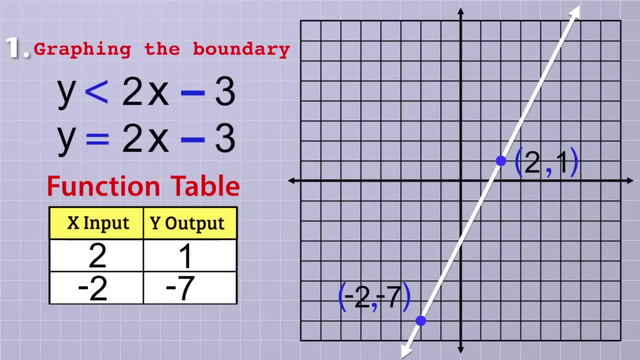 If x is 2, then y will be 1.. And if x is negative 2, then y will be negative 7.. Plotting those two points on the graph and then connecting the dots gives us this line, which is the boundary line of the inequality. But are the points exactly along that line? 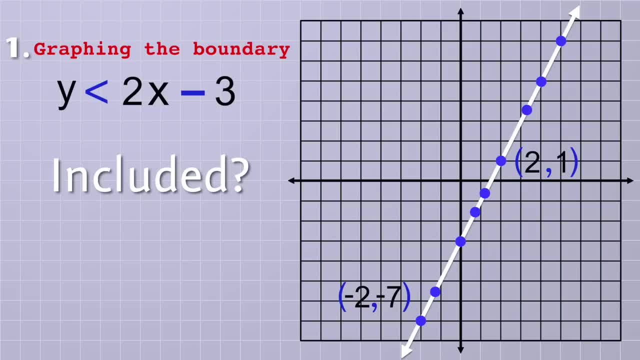 included in the solution set To answer that we need to check the inequality sign of the original problem. In this case, since we have the less than sign, that does not include the equal sign. the line itself won't be included in the set of valid answers, So we'll draw. 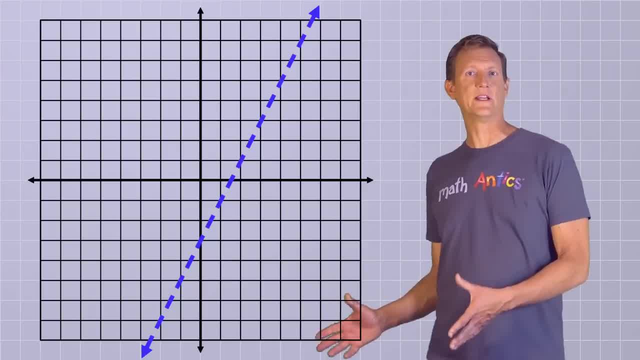 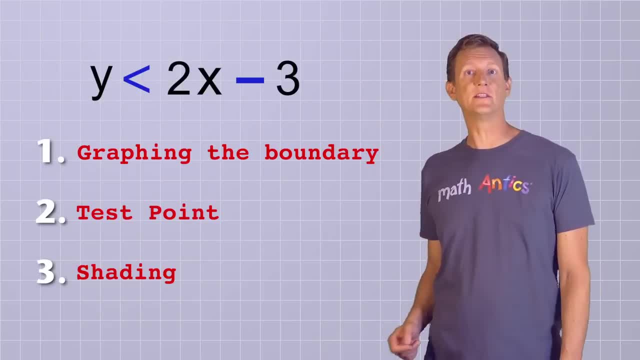 it with a dashed line instead of a solid line. Great, Now that we have our boundary line correct, we need to figure out which side of the line is in the answer set. To do that, we need to pick a test point, Because we know. 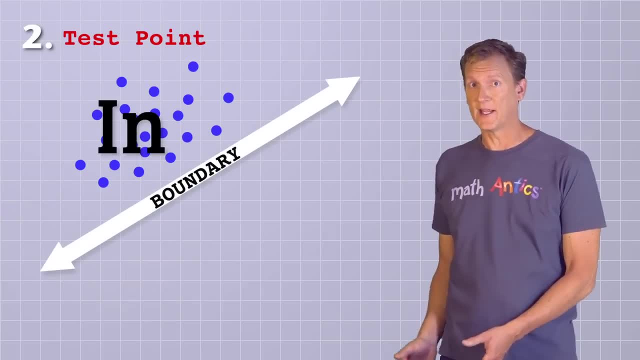 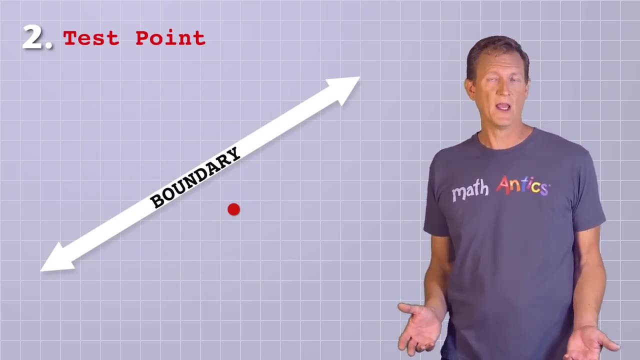 that all of the points on one side of the line are in the answer set and all of the points on the other side are not. we only need to know the status of one point to tell which side is which. In other words, if we can. 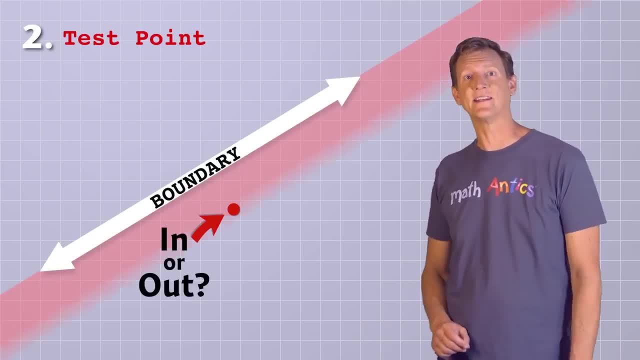 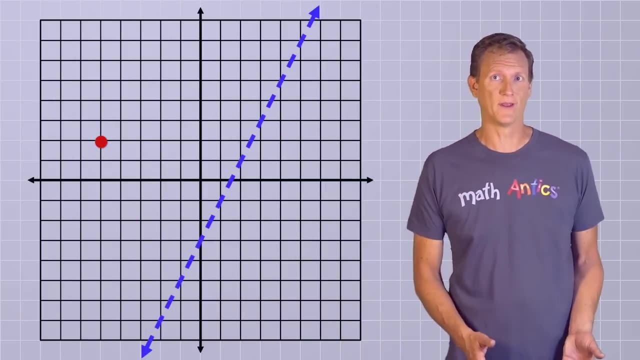 determine whether the test point is in or out. we'll know if that entire side is in or out. It doesn't matter where the test point is. so feel free to pick something really easy to work with. I mean, why pick something like negative 2.17 comma 3.59, when you can just 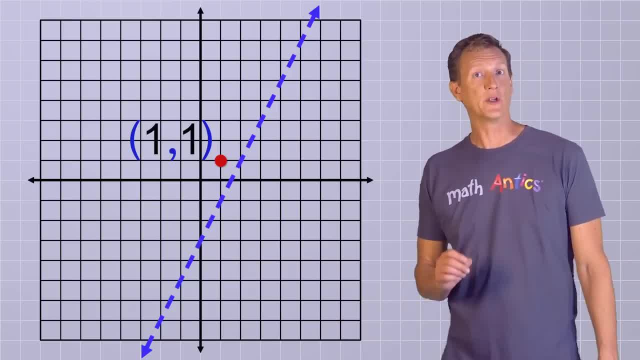 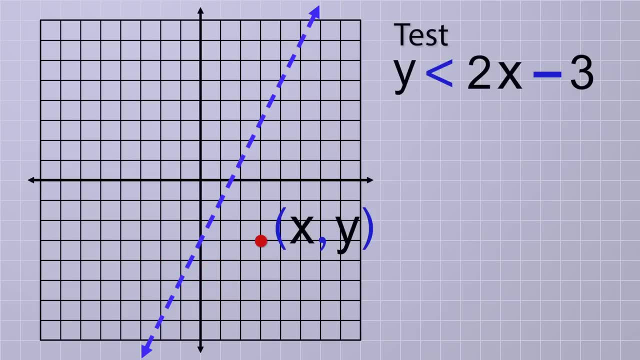 pick 0 comma 0 or 1 comma 1?? The only real restriction is that the test point can't be on the boundary line itself. Once you've decided which test point to try, plug its x and y values into the inequality and then simplify it. For example, if we pick the point 0 comma 0, we'd plug those. 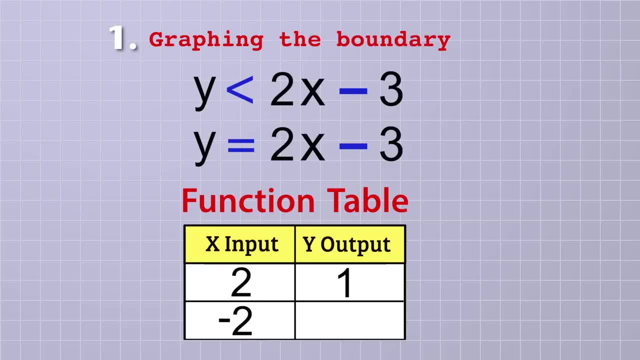 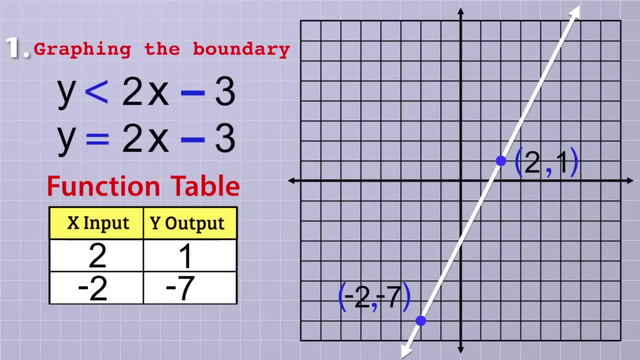 If x is 2, then y will be 1.. And if x is negative 2, then y will be negative 7.. Plotting those two points on the graph and then connecting the dots gives us this line, which is the boundary line of the inequality. But are the points exactly along that line? 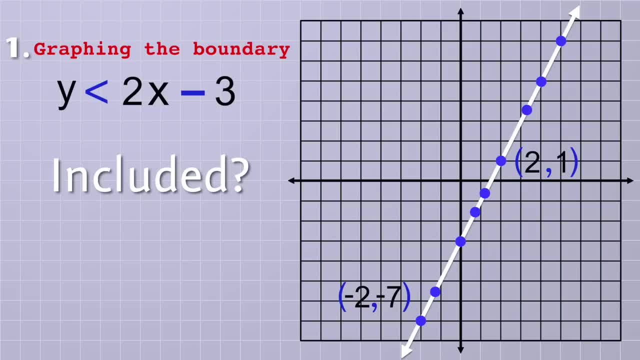 included in the solution set To answer that we need to check the inequality sign of the original problem. In this case, since we have the less than sign, that does not include the equal sign. the line itself won't be included in the set of valid answers, So we'll draw. 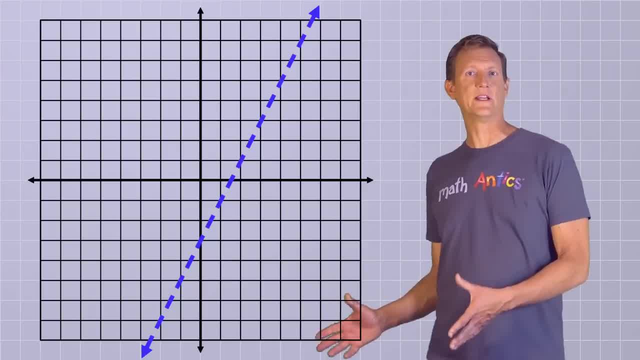 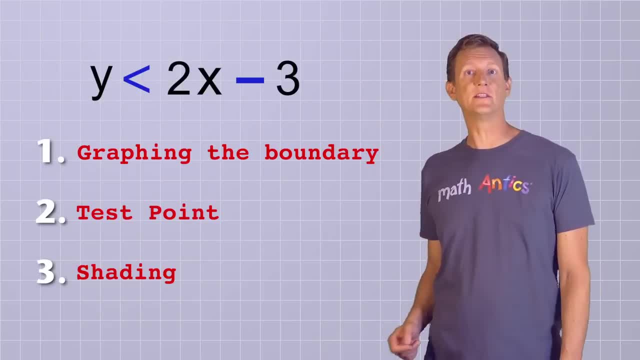 it with a dashed line instead of a solid line. Great, Now that we have our boundary line correct, we need to figure out which side of the line is in the answer set. To do that, we need to pick a test point, Because we know. 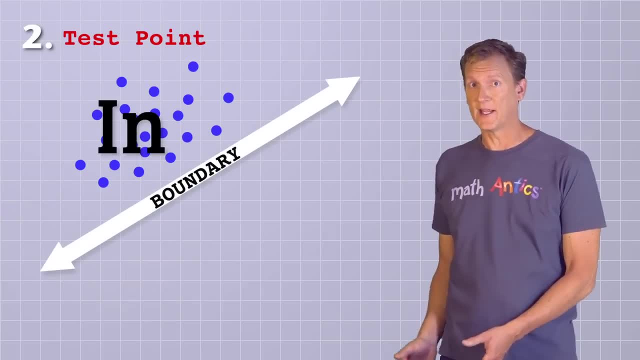 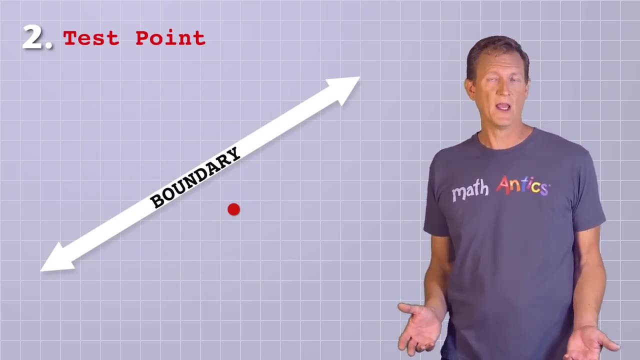 that all of the points on one side of the line are in the answer set and all of the points on the other side are not. we only need to know the status of one point to tell which side is which. In other words, if we can. 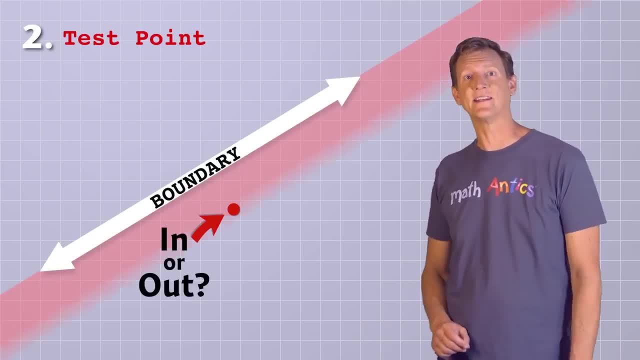 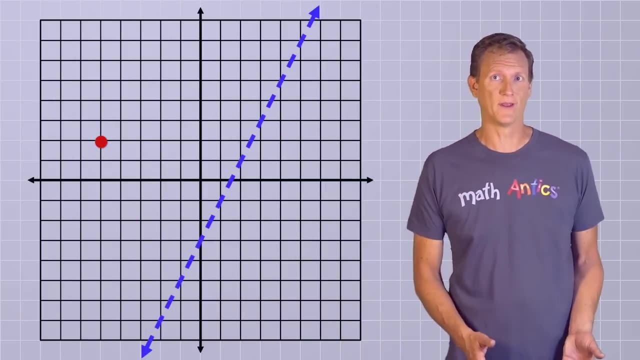 determine whether the test point is in or out. we'll know if that entire side is in or out. It doesn't matter where the test point is. so feel free to pick something really easy to work with. I mean, why pick something like negative 2.17 comma 3.59, when you can just 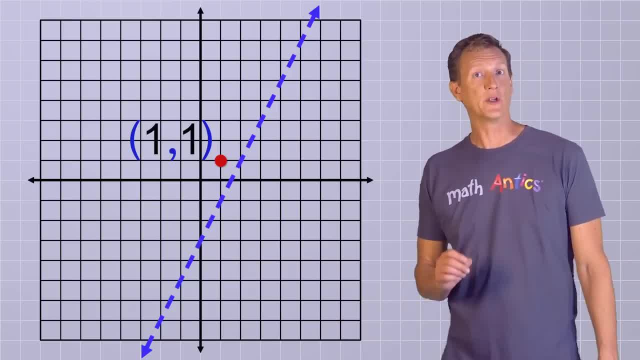 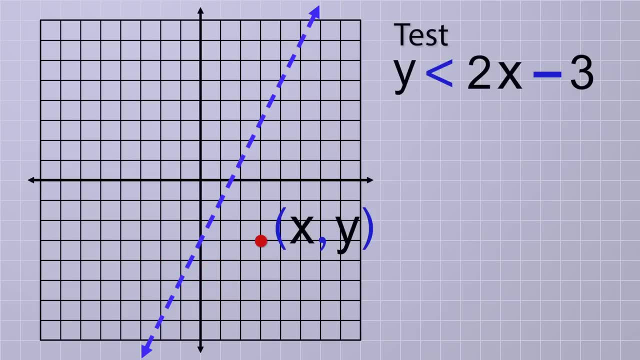 pick 0 comma 0 or 1 comma 1?? The only real restriction is that the test point can't be on the boundary line itself. Once you've decided which test point to try, plug its x and y values into the inequality and then simplify it. For example, if we pick the point 0 comma 0, we'd plug those. 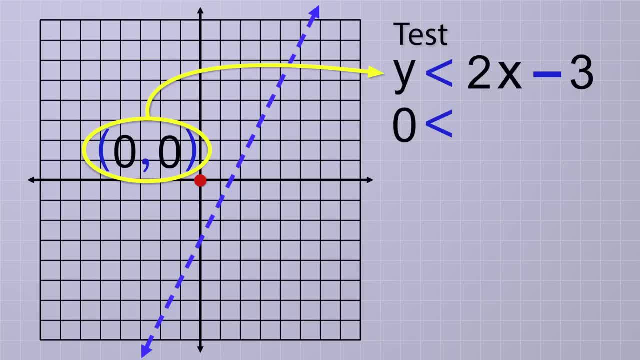 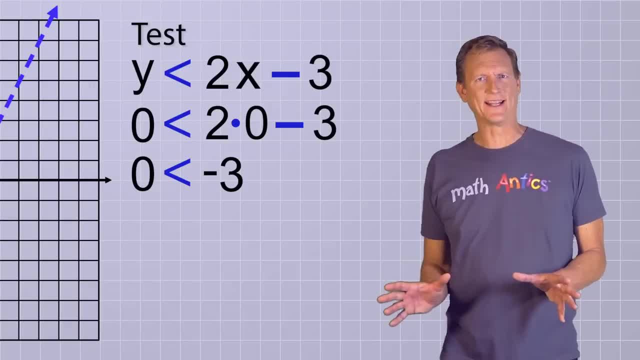 x and y values into the inequality to get: 0 is less than 2 times 0 minus 3, which simplifies to: 0 is less than negative 3.. But hold on a second… that's not true. 0 is NOT less than negative 3.. Ah, that's. 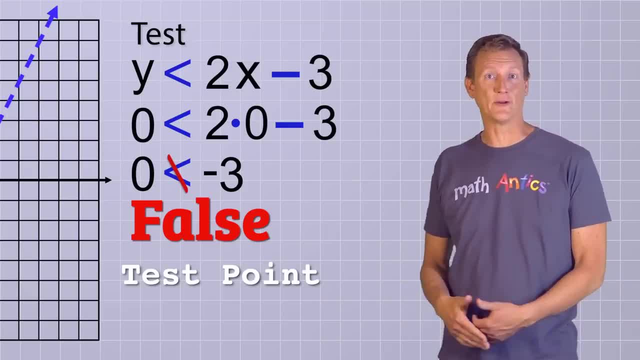 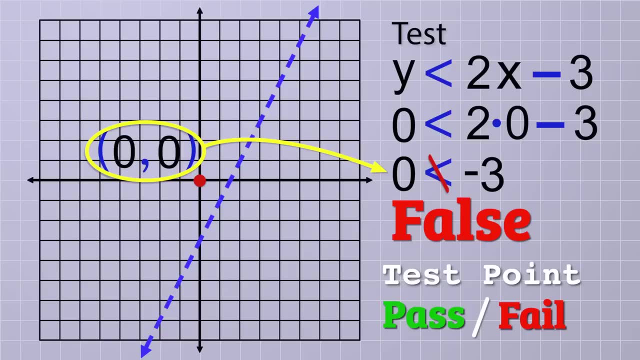 why it's called a test point. The point that you choose can either pass or fail the test. In this case, since plugging the points x and y values into the inequality, you can't do that. That means that the point is NOT a valid answer for the inequality. 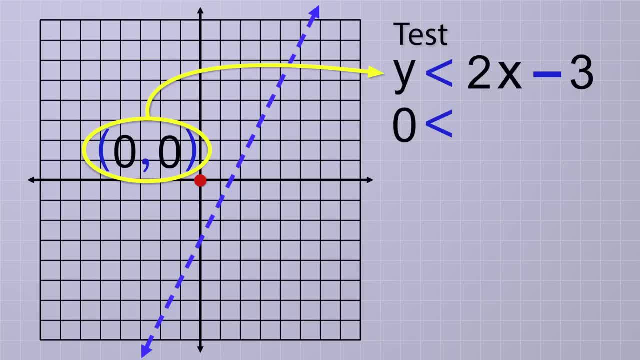 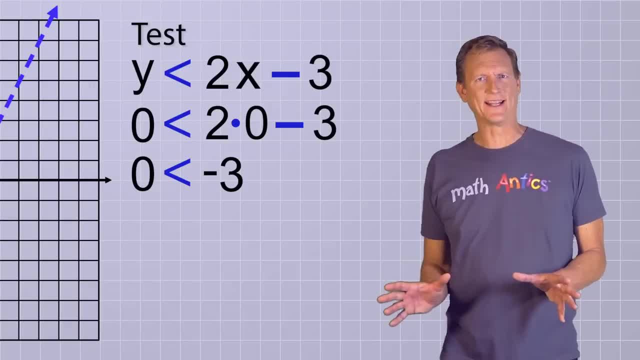 x and y values into the inequality to get: 0 is less than 2 times 0 minus 3, which simplifies to: 0 is less than negative 3.. But hold on a second… that's not true. 0 is NOT less than negative 3.. Ah, that's. 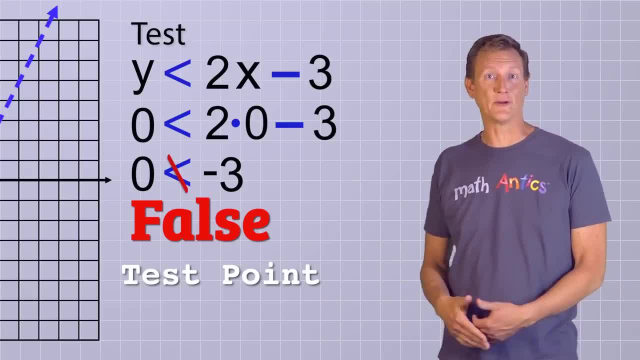 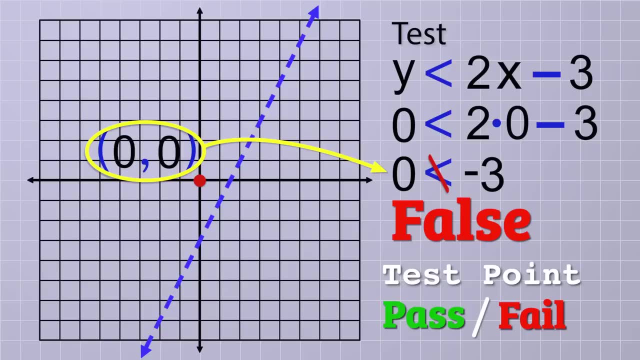 why it's called a test point. The point that you choose can either pass or fail the test. In this case, since plugging the points x and y values into the test point is a test, that means that the point is NOT a valid answer for the inequality. Therefore, 0 comma. 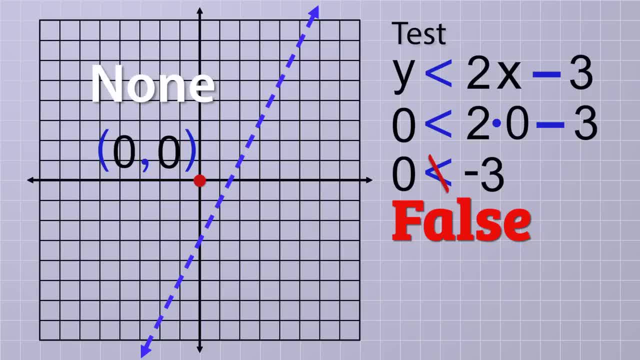 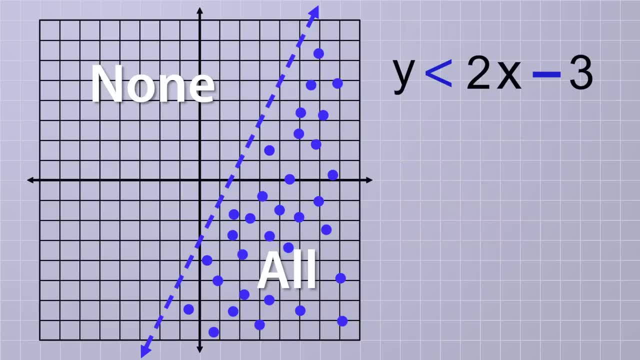 0 must be on the side of the boundary line where NONE of the points are included in the solution set, which means that all of the points on the other side WILL be included. So that brings us to the last step. We just need to shade the correct side of the line. 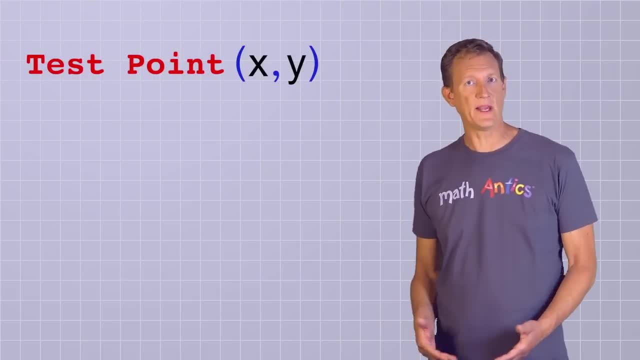 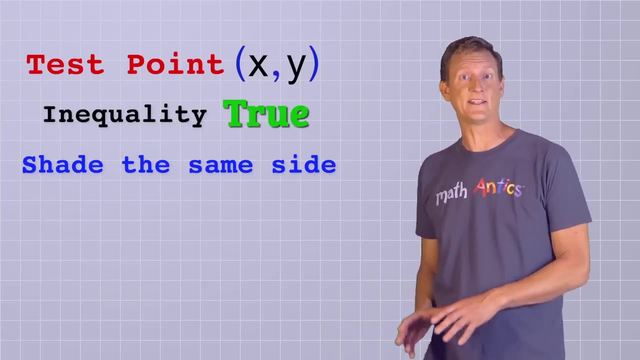 like so. To summarize, if the test point you pick makes the inequality true, then you've picked a point that's in the answer set, which means that you'll shade the same side of the graph that that test point is on. But if the test point gives you a FALSE statement, 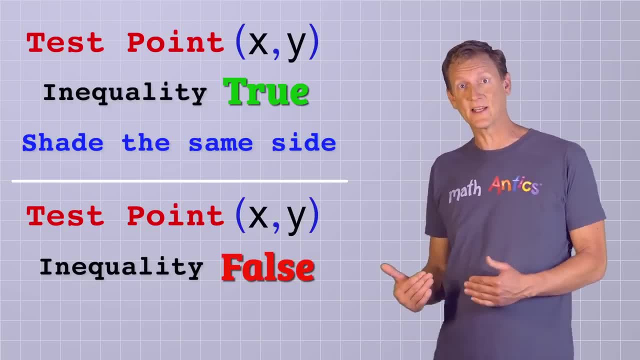 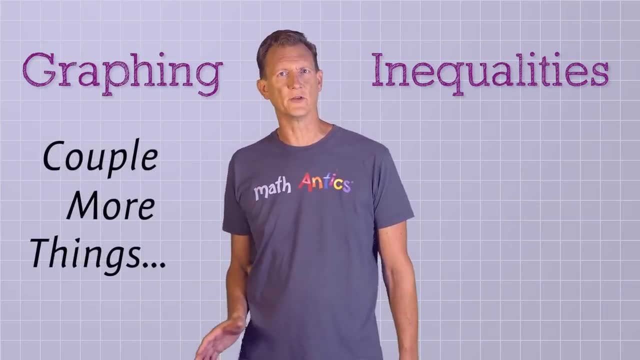 then you know that it's NOT in the answer set, which means that you'll leave that side blank and shade the other side. So that's the basics of graphing inequalities, But there's a couple more things that you'll need to know to be successful at it. After all, not every inequality that you encounter 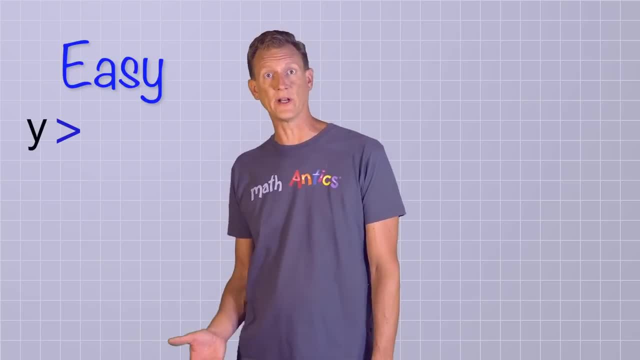 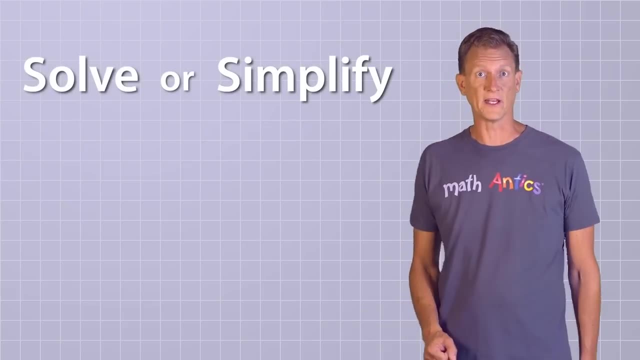 will be in a nice, easy-to-work-with form like y is greater than mx plus b. You may have a few things that need to be simplified. Fortunately, you can solve or simplify inequalities almost the same way that you do with equations. All of the same principles apply, like combining. 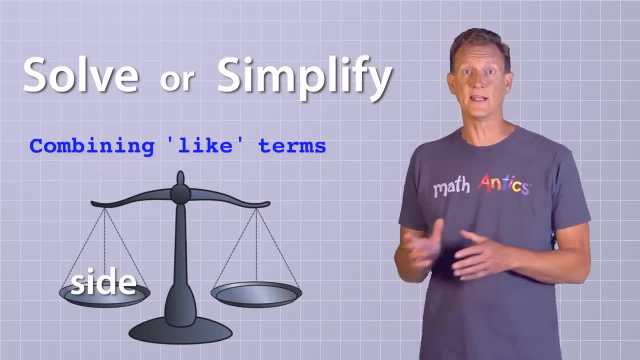 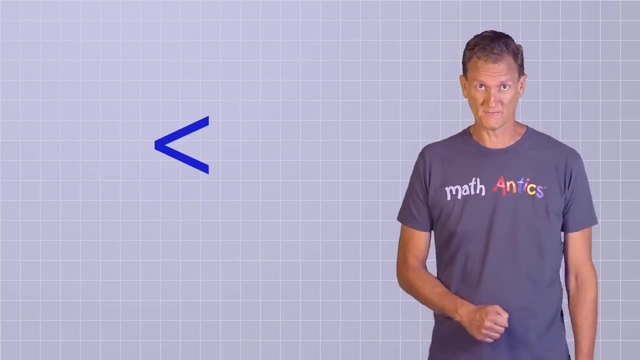 like terms and the idea that anything you do to one side needs to be done to the other side too. However, there are a couple situations where you need to FLIP the inequality sign. You never had to worry about that with equations, because order doesn't matter when both sides 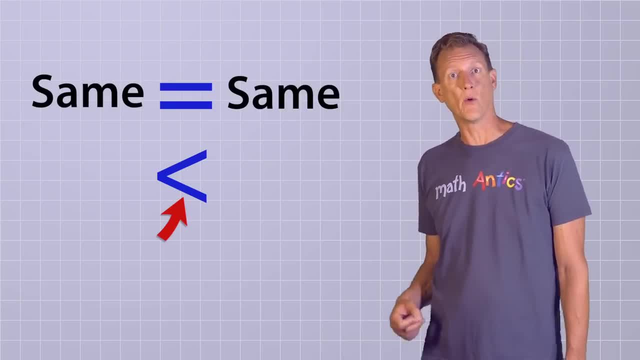 have the exact same value, But inequalities tell us that one side has the same value as the other side, so you don't have to worry about that. One side has a greater value than the other, and the open end of the inequality sign always. 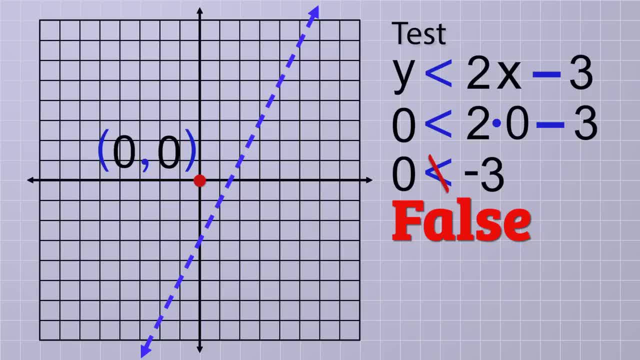 Therefore, 0 comma 0 must be on the side of the boundary line where NONE of the points are included in the solution set, which means that all of the points on the other side WILL be included. So that brings us to the last step. We just need to shade the correct side. 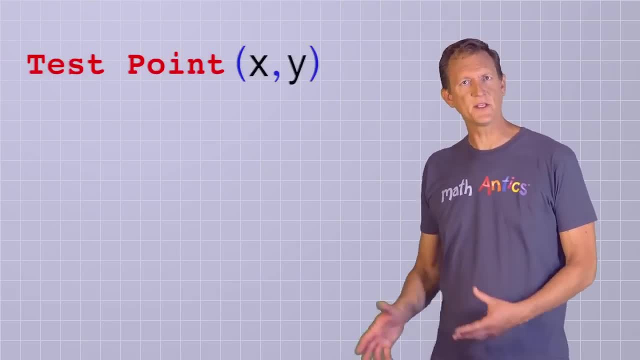 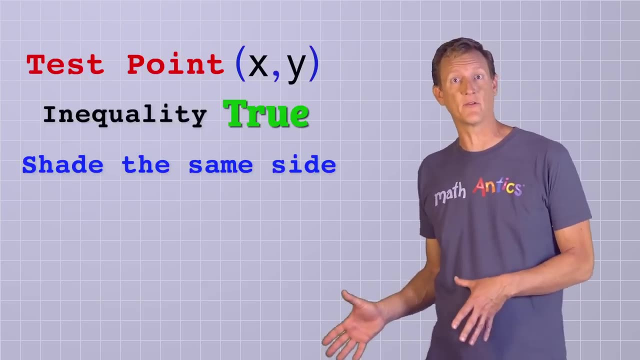 of the line like so: To summarize: if the test point you pick makes the inequality true, then you've picked a point that's in the answer set, which means that you'll shade the same side of the graph that that test point is on. But if the test point gives you a FALSE statement, 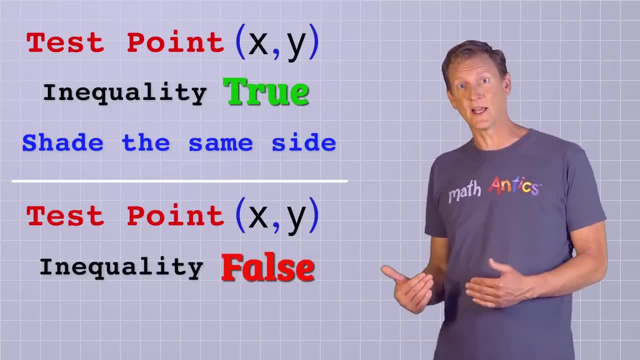 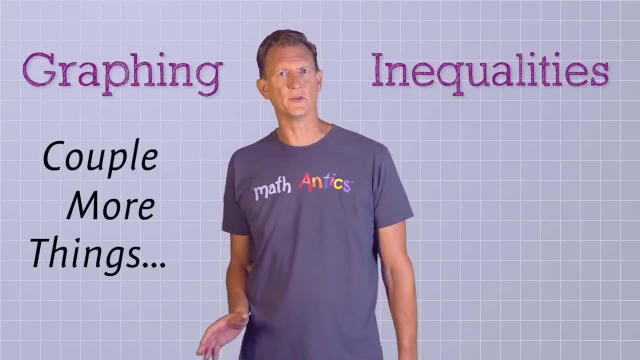 then you know that it's NOT in the answer set, which means that you'll leave that side blank and shade the other side. So that's the basics of graphing inequalities, But there's a couple more things that you'll need to know to be successful at it. After all, not every inequality that you encounter 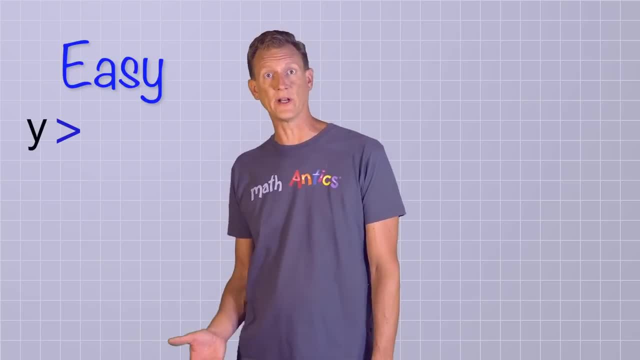 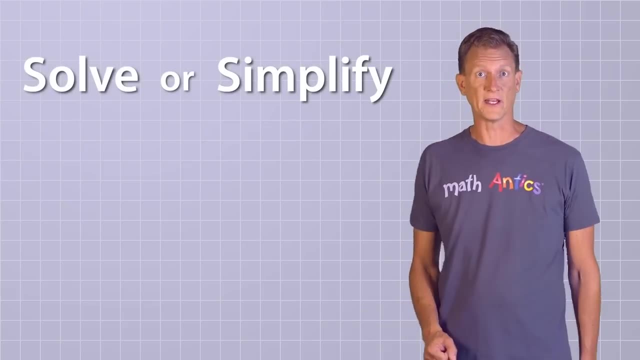 will be in a nice, easy-to-work-with form. like y is greater than mx plus b. You may have a few things that need to be simplified. Fortunately, you can solve inequalities almost the same way that you do with equations. All of the same principles apply, like combining. 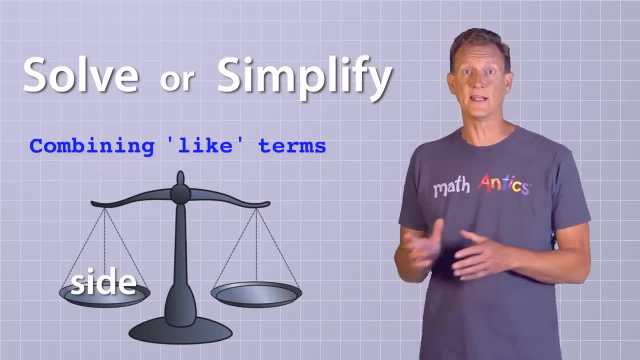 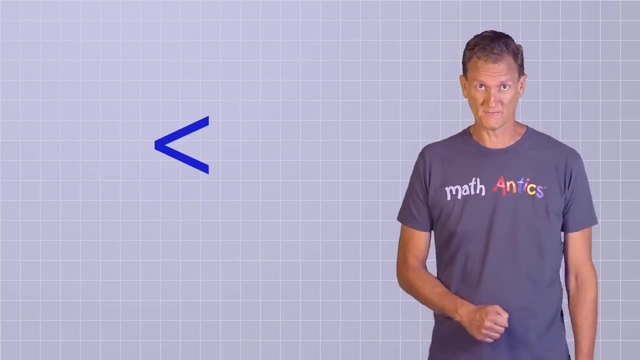 like terms and the idea that anything you do to one side needs to be done to the other side too. However, there are a couple situations where you need to FLIP the inequality sign. You never had to worry about that with equations, because order doesn't matter when both sides 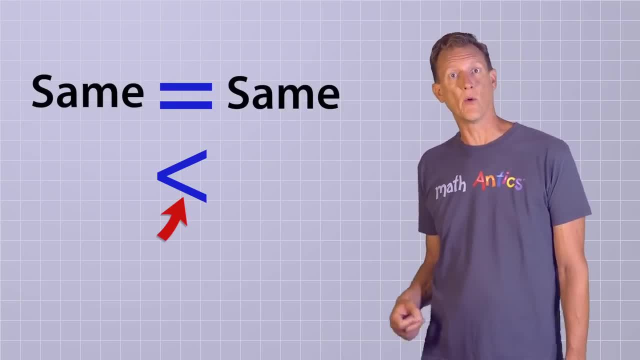 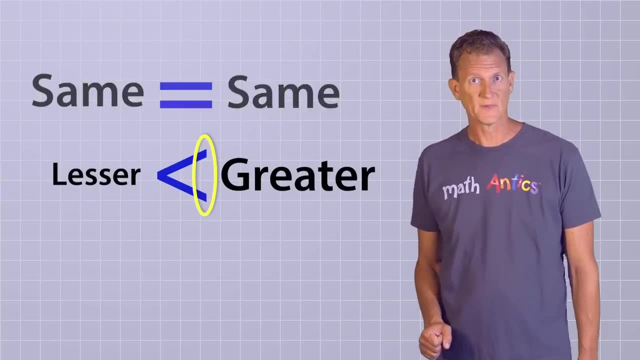 have the exact same value, But inequalities tell us that one side is equal to the other side. One side has a greater value than the other and the open end of the inequality sign always faces that greater side. That means that if you need to switch the left and right sides, 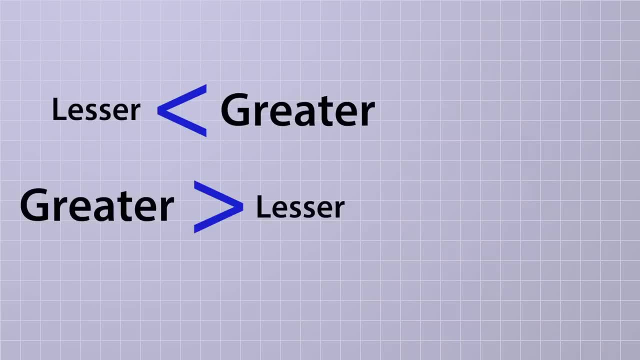 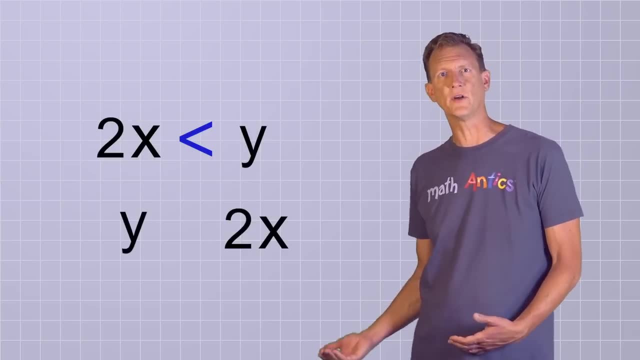 of an inequality, you also need to switch the inequality sign. For example, if you have the inequality 2x, y and you want it to rearrange so that y comes first, you'd need to flip the inequality sign when you do that. So just remember, if you switch the sides, switch. 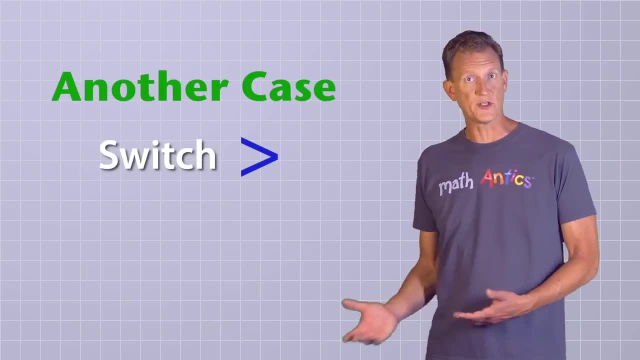 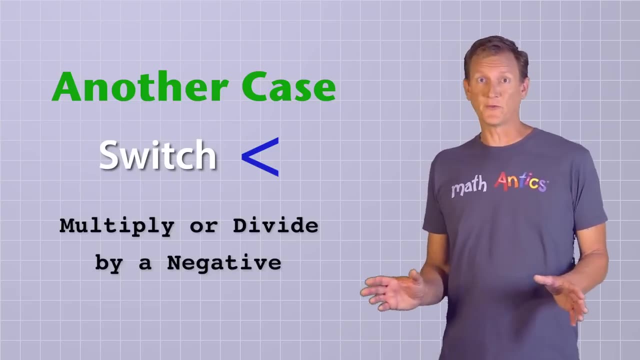 the inequality sign. Another way to switch the inequality sign is whenever you multiply or divide both sides by a NEGATIVE number or term. You don't need to do this for any other operations. You can add or subtract positive or negative terms from both sides and you can multiply. 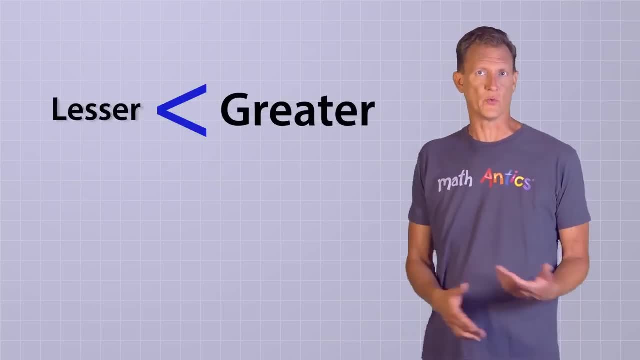 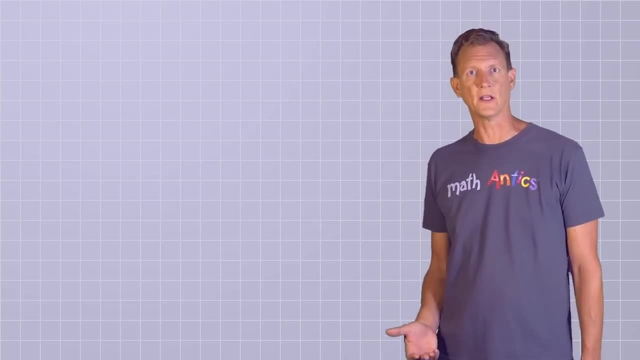 faces that greater side. That means that if you need to switch the left and right sides of an inequality, you also need to switch the inequality sign. For example, if you have the inequality 2x- y and you want it to rearrange so that y comes first, you'd need to flip. 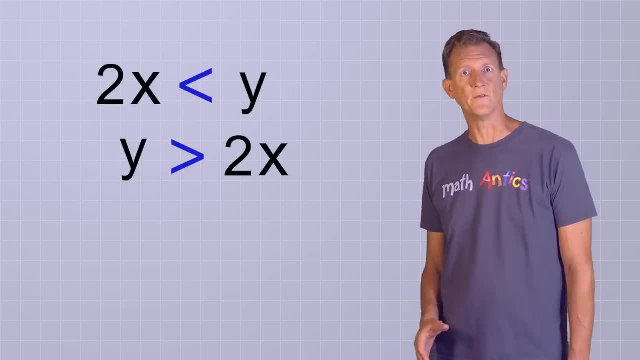 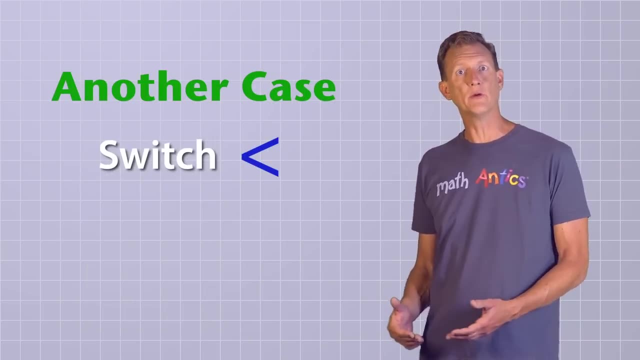 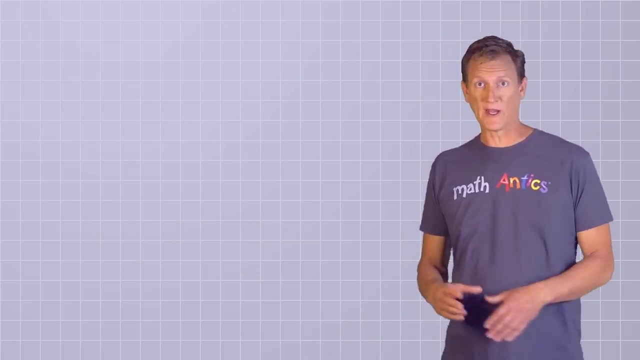 the inequality sign when you do that. So just remember, if you switch the sides, switch the inequality sign. Switch the inequality sign is whenever you multiply or divide both sides by a negative number or term. You don't need to do this for any other operations. You can add or subtract. 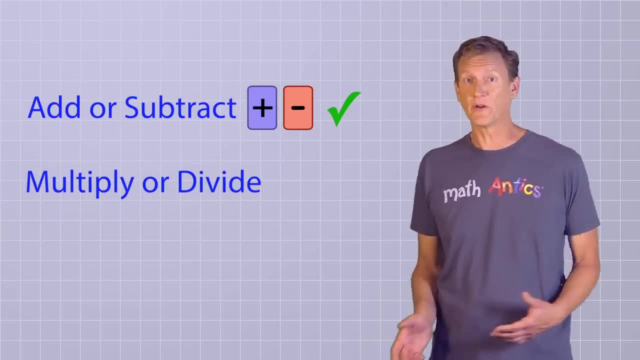 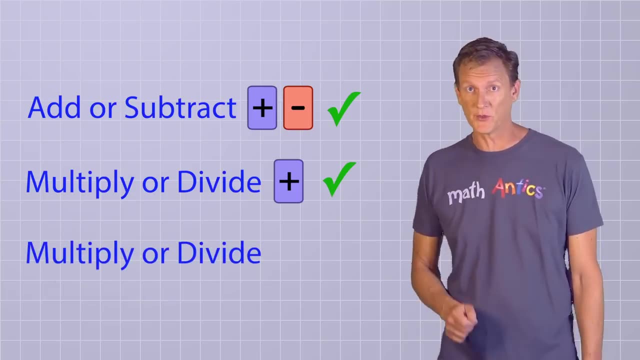 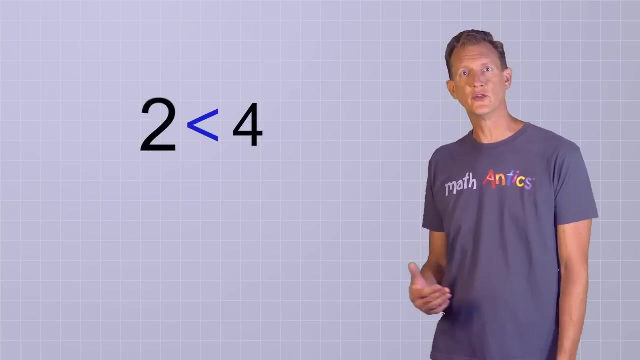 positive or negative terms from both sides and you can multiply or divide both sides by a positive term without needing to switch the inequality sign. It's only when you multiply or divide both sides by a negative that you need to flip it To understand why that's necessary. have a look at the simple inequality: 2 is less than 4, and imagine: 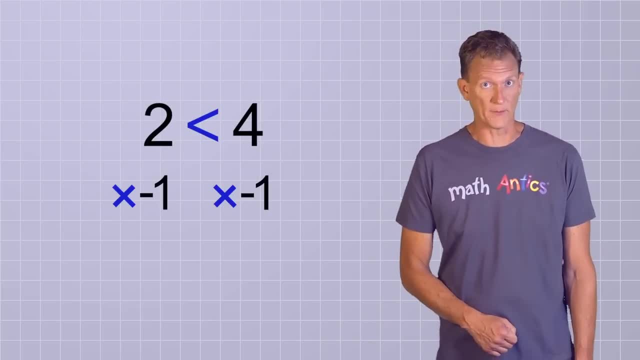 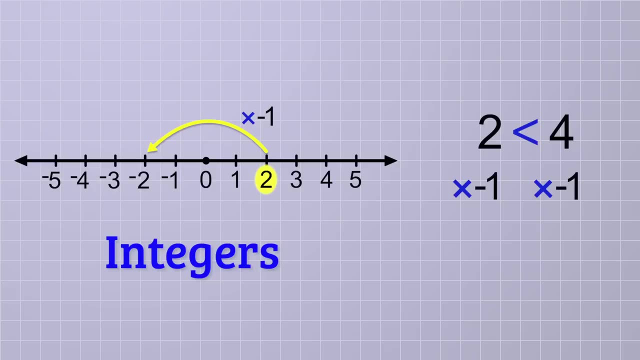 what would happen if you multiplied both sides by negative 1.. In a previous video about integers you learned that multiplying by negative 1 switches a number to the opposite side of the number line and vice versa. Doing that to two different numbers actually changes their order. Positive 2 is less than 4, but negative 2 is greater. 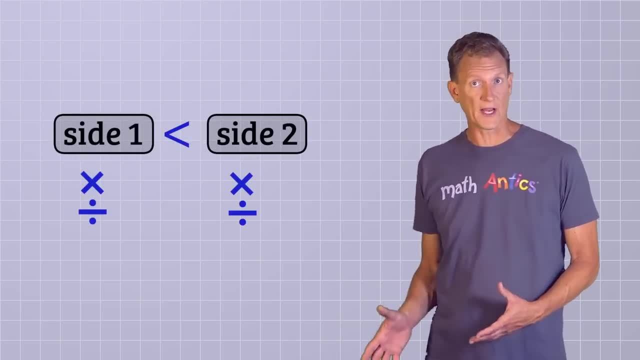 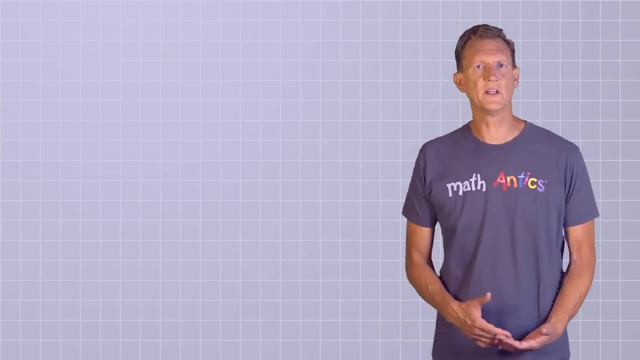 than negative 4.. That's why every time you multiply or divide both sides of an inequality by a negative, you NEED to switch the inequality sign. For example… Suppose you're given the inequality, negative, 2y plus 1 is greater than x plus 5, and you 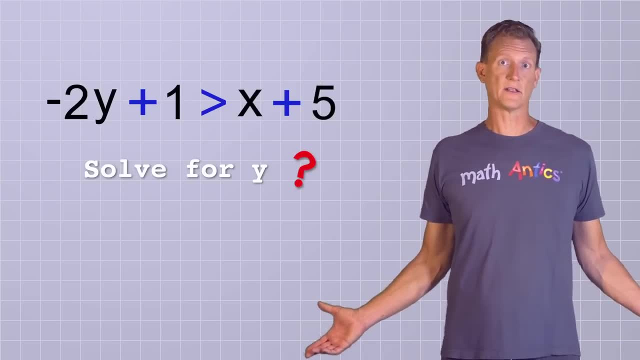 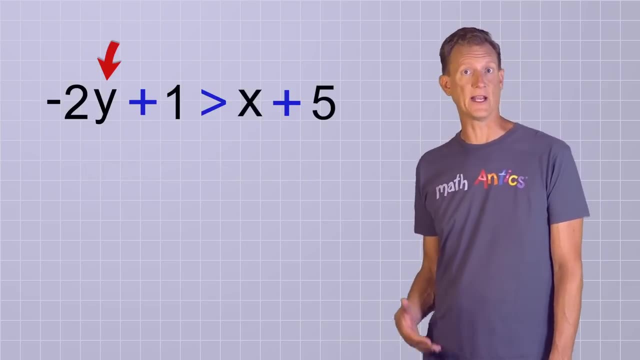 need to solve it for y before you graph it. How would you do that? Well, we want to get y all by itself, but two things are currently being done to it: It's being multiplied by negative 2, and 1 is being added to that term. 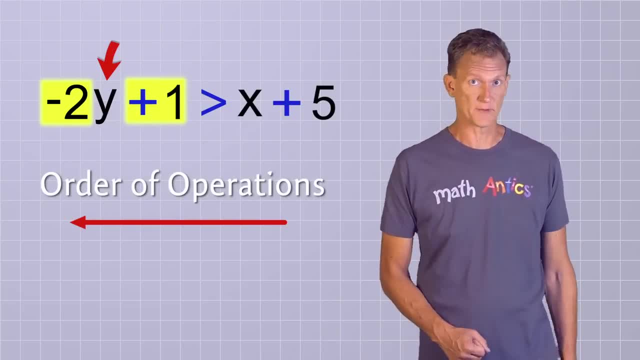 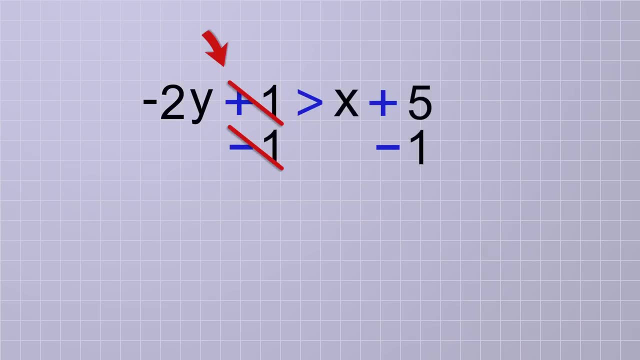 Let's undo those operations using order of operations in reverse. First we'll subtract 1 from both sides: On the left side the plus 1 and the minus 1, cancel out, leaving just negative 2y. And on the right side the x plus 5 minus 1. simplifies. 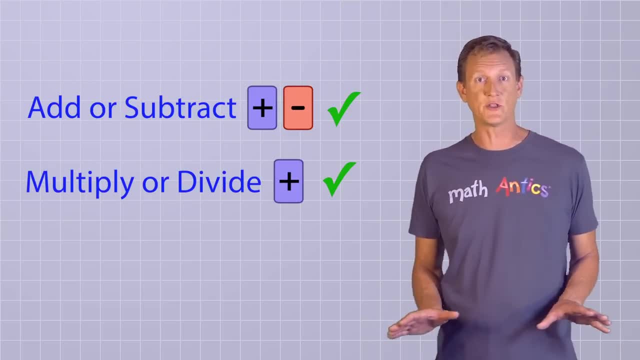 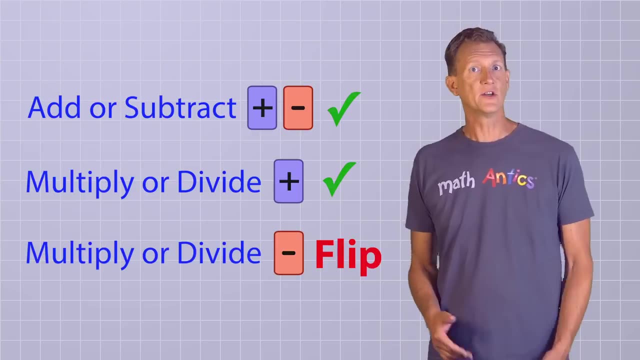 or divide both sides by a positive term without needing to switch the inequality sign. It's only when you multiply or divide both sides by a negative that you need to flip it To understand why that's necessary. have a look at the simple inequality: 2 is less. 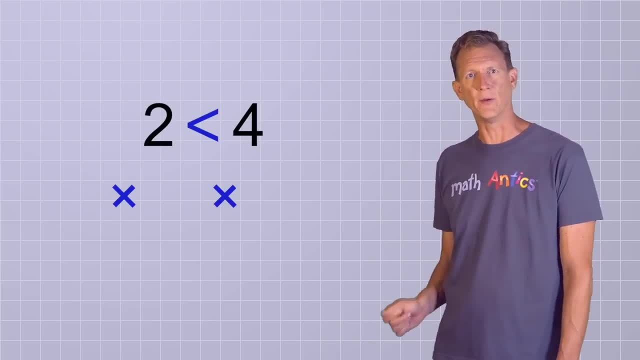 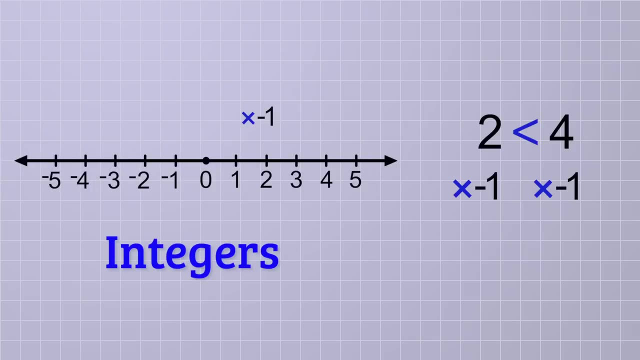 than 4.. What would happen if you multiplied both sides by negative 1?? In a previous video about integers, you learned that multiplying by negative 1 switches a number to the opposite side of the number line and vice versa, Doing that to two different. 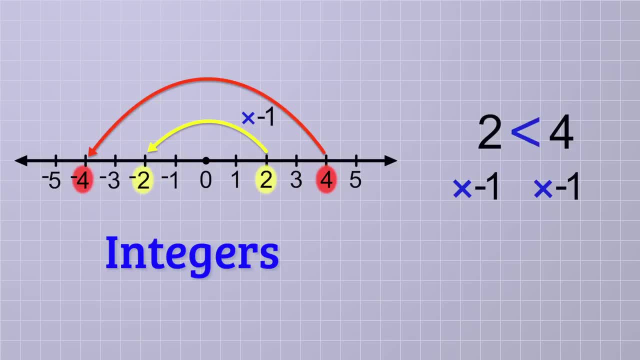 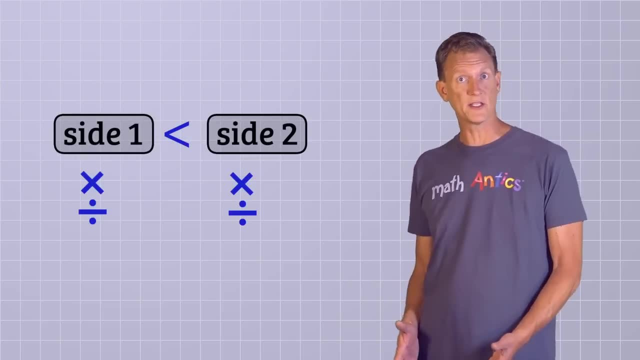 numbers actually changes their order. Positive 2 is less than 4, but negative 2 is greater than negative 4.. That's why, every time you multiply or divide both sides of an inequality by a negative, you NEED to switch the inequality sign. 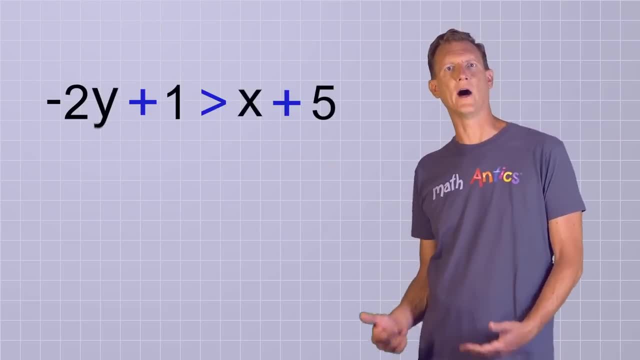 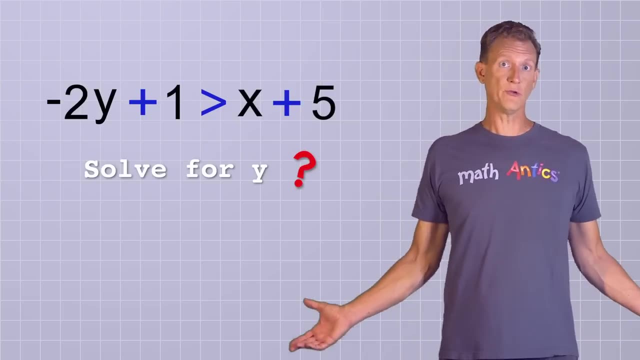 For example, Suppose you're given the inequality negative, 2y plus 1 is greater than x plus 5, and you need to solve it for y before you graph it. How would you do that? Well, we want to get y all by itself, but two things are currently being done to it. 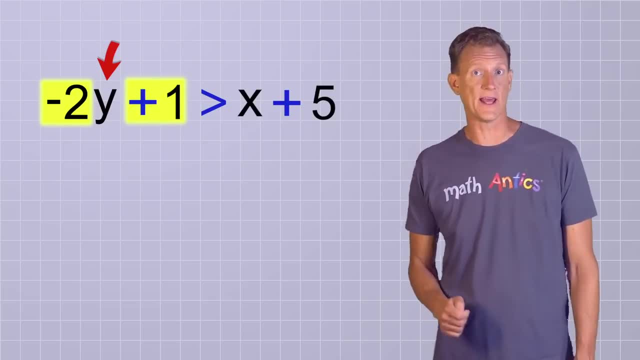 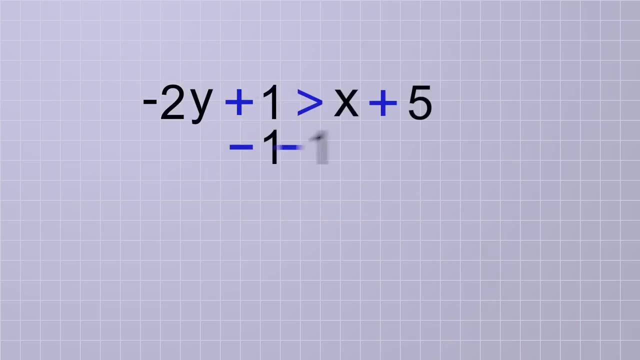 It's being multiplied by negative 2, and 1 is being added to that term. Let's undo those operations using order of operations in reverse. First we'll subtract 1 from both sides: On the left side the plus 1 and the minus. 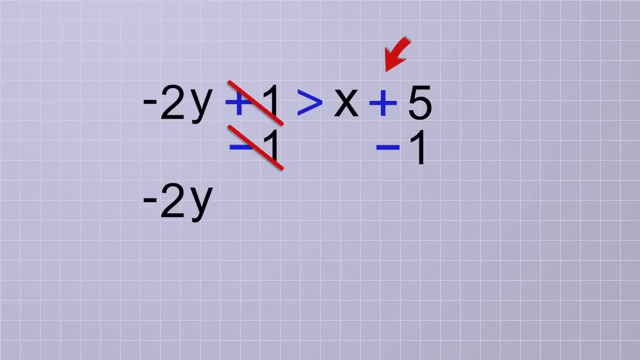 1 cancel out, leaving just negative 2y. And on the right side the x plus 5 minus 1 simplifies to x plus 4.. Notice, we didn't switch the inequality sign when we did that operation. It's still the greater than sign. 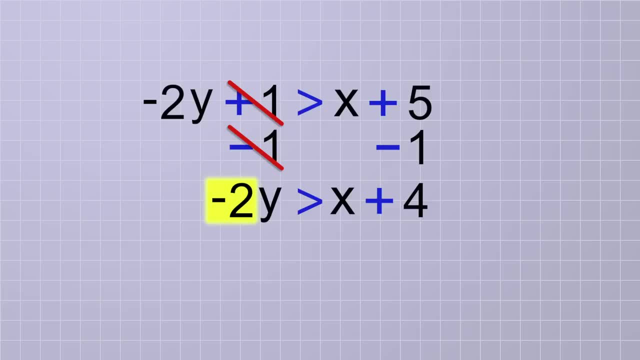 But now we need to get rid of the negative 2 that's being multiplied by y. That can be done by dividing both sides by negative 2.. Because that will change the sign of both sides. we do need to flip the inequality sign for this operation. It was the greater than sign originally, but now it's the greater than sign. 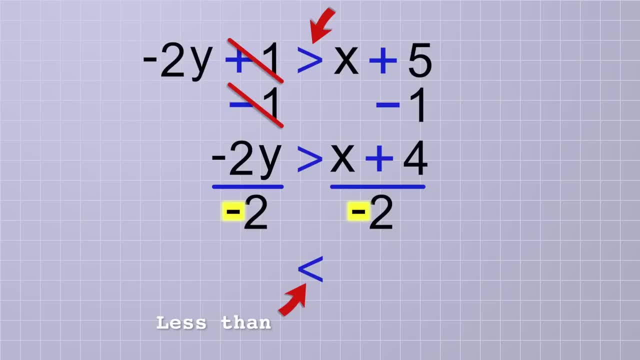 It was the greater than sign originally, but now it's the greater than sign. It was the greater than sign originally, but now it's the greater than sign. But now it will become the less than sign. On the left, the negative 2 over negative 2 cancel, leaving positive y all by itself.